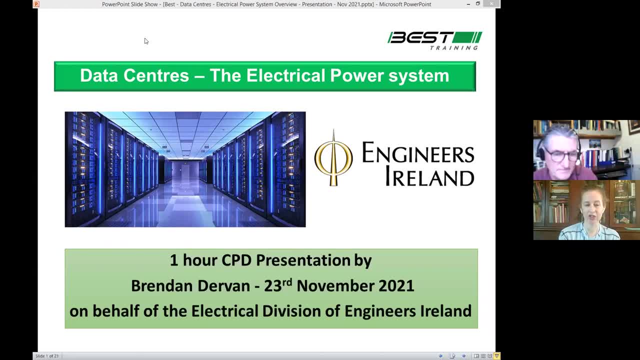 engineering data centres. Brendan, as I said, conducts a number of CPD training courses and you can visit wwwbesttrainingie for further information or keep an eye on the Engineers Ireland website. Thank you again, Brendan, in advance and over to you, Thanks very much for that. 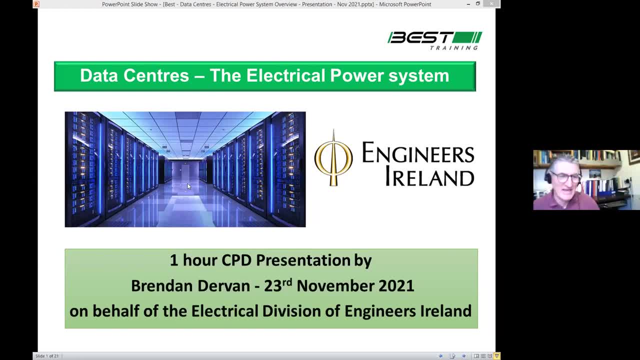 introduction, Arla, and nicely summed up: Okay folks, thank everybody, for we've a great, great turnout here today, so thanks to everybody for taking the time out to listen to this presentation. It's actually headlines in the Irish Times this morning: data centres and the whole issue with 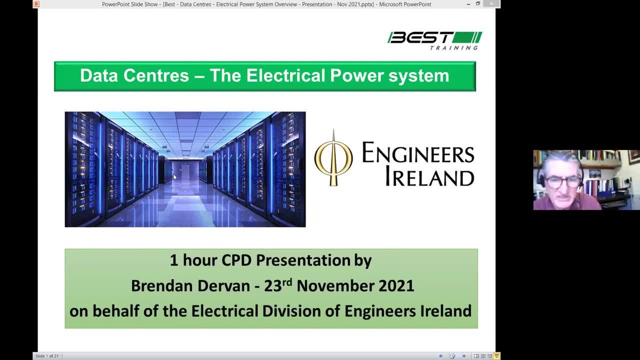 connectivity onto the grid and grid congestion and all these issues. so what we're going to look at today is the electrical system from literally from the pylon into the back of the server rack. so what we're looking at here in this image actually is inside a typical data hall and there 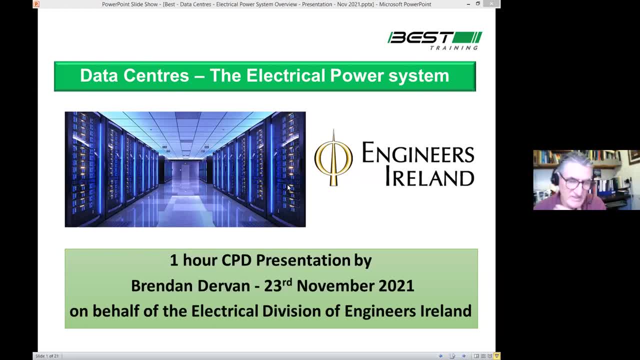 are the server racks, and within them you can see those rows and rows of servers stacked up, which so each of those racks could be typically drawing 20-30 kilowatts of power, and that converts into heat, and that heat has to be dissipated, so that's where all the power goes, in the data centre. So 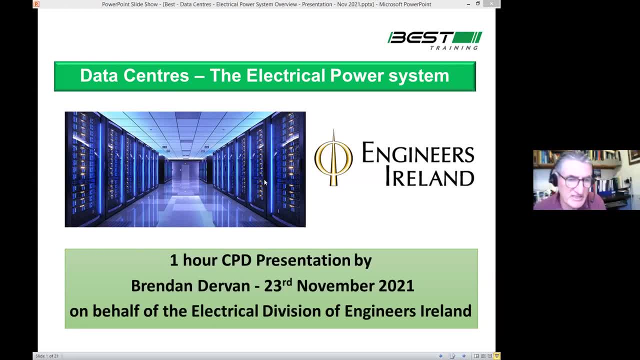 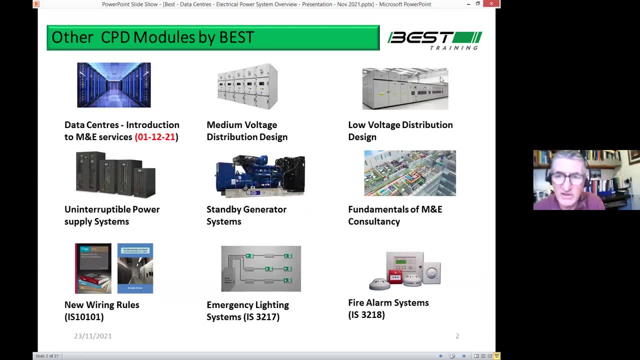 we're going to look today at the journey from the pylon right into the back of the server cabinets. So Arla mentioned earlier on that I've retired and it's kind of semi-retirement because I've taken up this role of trainer over the last two. 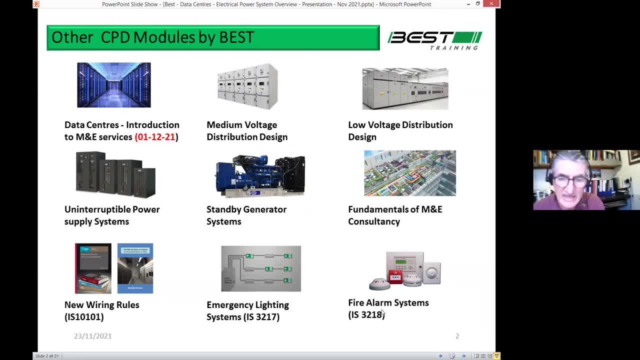 three years and I've developed a number of courses, and the reason is I'm kind of passionate about engineering, particularly electrical engineering. that was my field and I feel I haven't spent 40 years in the industry. it's worth sharing that knowledge there's there's a need for. 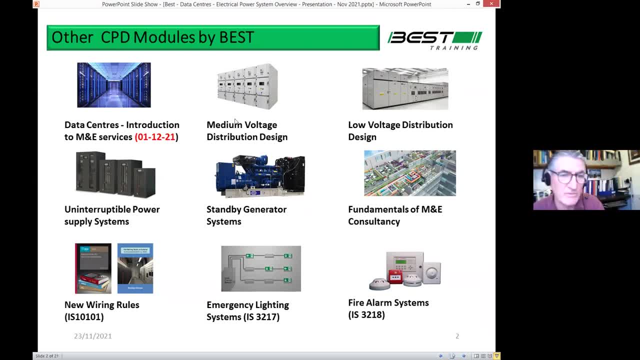 it and I like doing it, so it's kind of not really like work as such. so I initially developed one main training course on data centres and I kind of was going to leave it at that because there was a big demand for that, and then I developed the 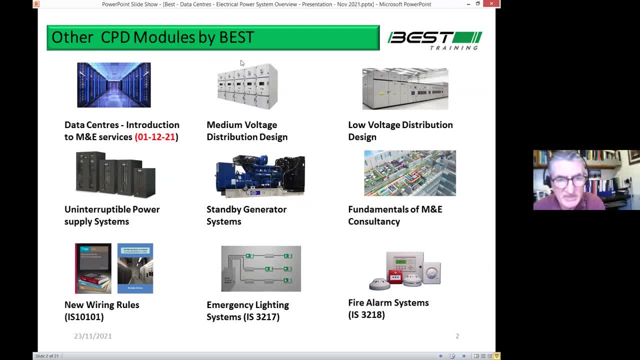 medium voltage course, which there's a big need in that area. there's a big knowledge gap, I suppose, in the building service industry, and I developed a course in that and then, of course, logically followed through on to develop a low voltage distribution course as well, and then I followed. 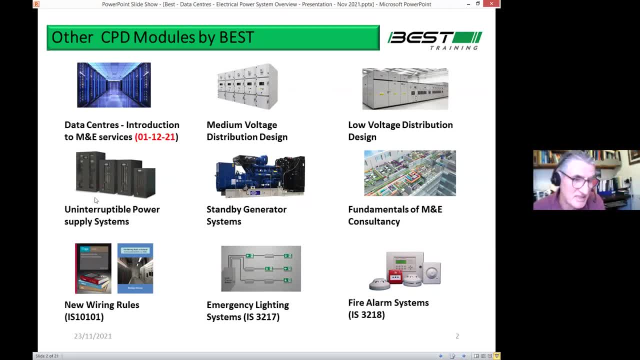 off to fill the suite on the data centre. I said you know uninterruptible power supply systems, or UPS as they're better known. I've a course on that and then one on standby generators and that's really the whole. those five courses is the real data centre suite of courses and, incidentally, I've highlighted in red, just so I. 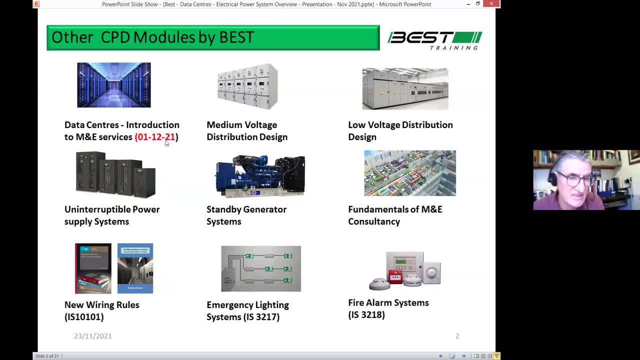 wouldn't forget it- and I nearly did, Orla has mentioned it- that the next day for the data centre course is on the 1st of December, Wednesday week. it's a really, really popular course. it's regularly booked out, fully booked out. it's very, very popular. it covers and all aspects of M&E. 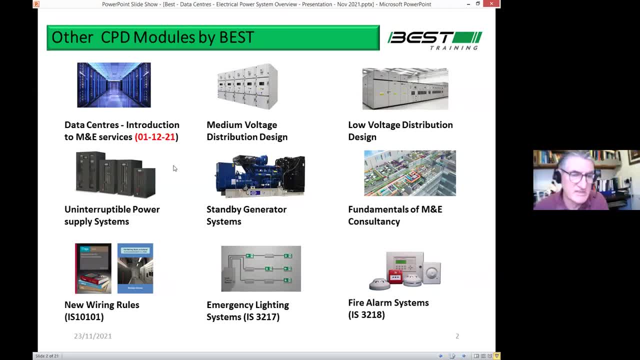 services. obviously the main focus will be on the power and cooling systems and very, very popular. so if you want you can, I'll remind you of it later at the end. you can book that directly with Engineers Ireland. do the course I do are fundamentals of M&E consultancy, which I 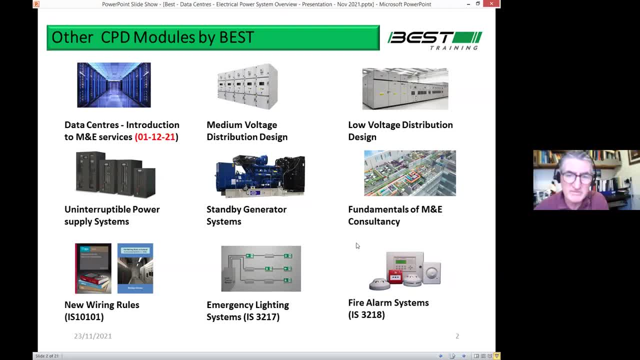 developed for people coming into the industry and coming out, because people are coming into the building service industry from all different career paths now and it's just to, I suppose, to praise them on the different aspects of what a consultant actually does. the most popular course by far is this bottom left hand one, the new wiring rules. 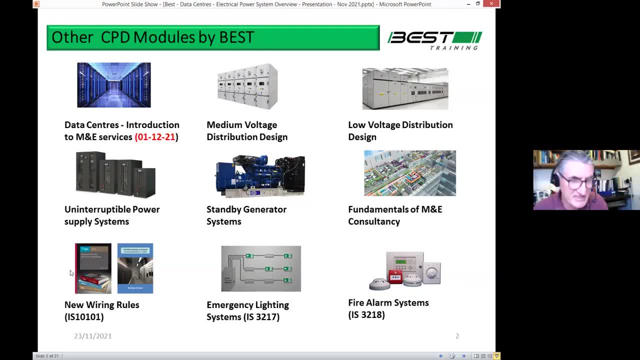 in in December, in February of this year, and so all new installations have to be designed to the new standard here, which is the bottom left hand image and the book beside it is my own guidebook which I just published. so I'm not, I'm not here to plug that, but just to let you know and that's a. 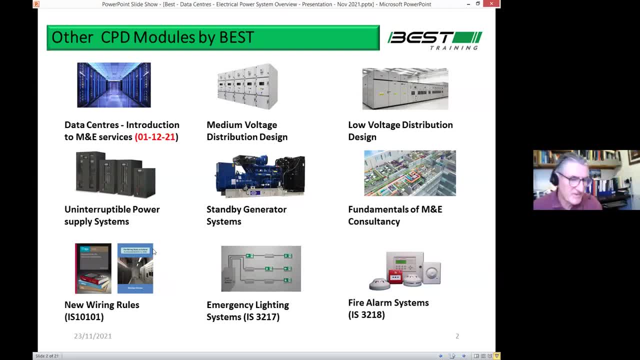 guidebook. it's a kind of um. it kind of demystifies the wiring rules. they're very, very difficult to read and understand, find your way around them, et cetera. so the book actually goes through the entire wiring rules and explains them in in their language I suppose, with lots of diagrams and charts and things like that. 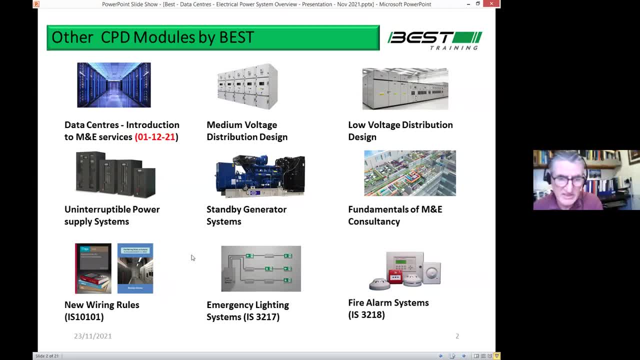 I'll do the two courses. I'm working on those at the moment. I'll be developing those in the coming weeks. the standards for emergency light and fire alarm are also going to be updated and changed significantly. so I'll be developing courses on these which hopefully I'll be running. 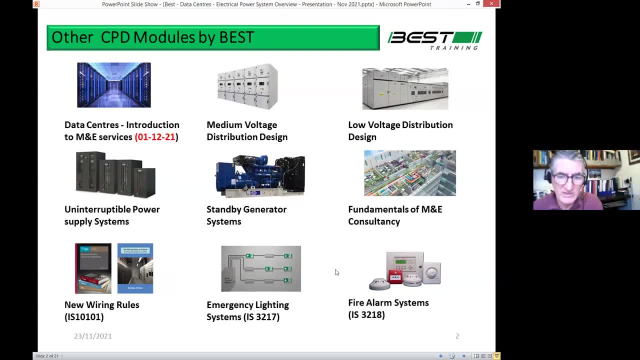 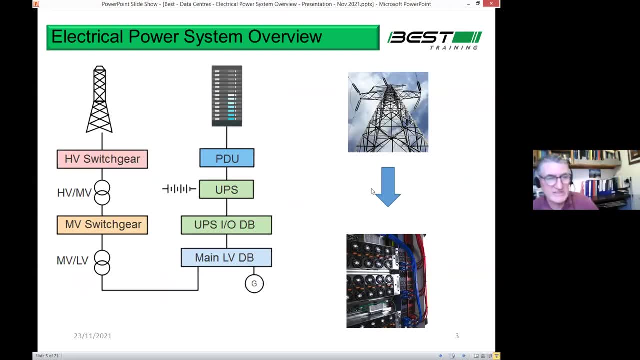 through Engineers Ireland again next year. so without further ado, I'll jump straight into today's topic, which is the electrical power system in data centers. so this little graphic is actually going to sum up what we're going to be talking about today. so obviously we take power from the 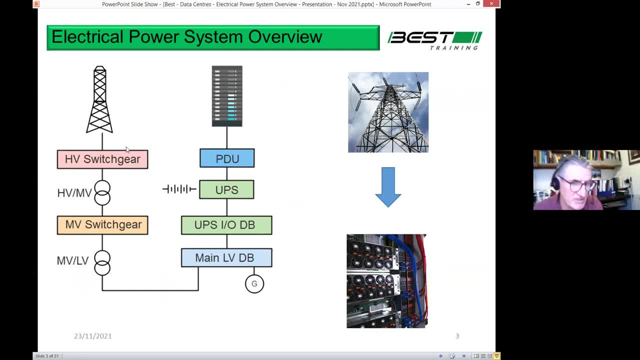 transmission Grid and it comes through HV switch gear, high voltage switch, which is usually owned by the ESB. then we transform down through the transformer here from high voltage down to medium voltage. now, this whole aspect of it, the connection to the transmission system, the high voltage which 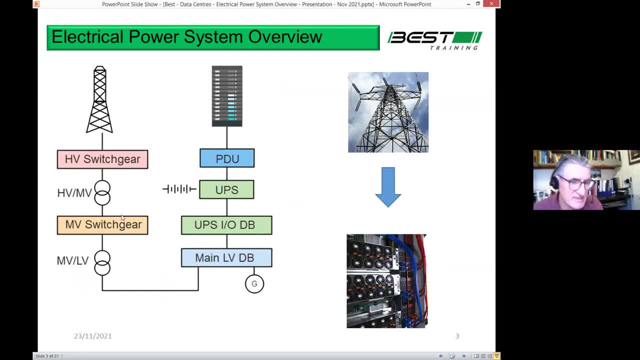 gear and the high voltage transformer. it's usually done as a specialist contract outside of the the normal building services contracts. so the normal building service engineer that designed the electrical system in the data center doesn't very often get involved in this, And I won't be either, because it's not my area of. 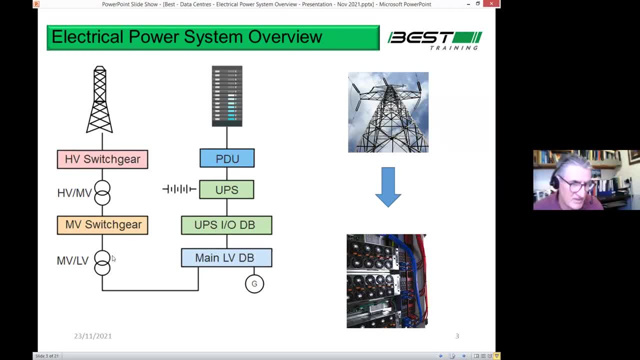 expertise. It's really from here down, from the MV switchgear downwards, that the electrical engineer on the data center gets involved in. So the first thing is the MV switchgear, or medium voltage switchgear. Medium voltage is above 1,000 volts up to 35,000 volts. So in Ireland, 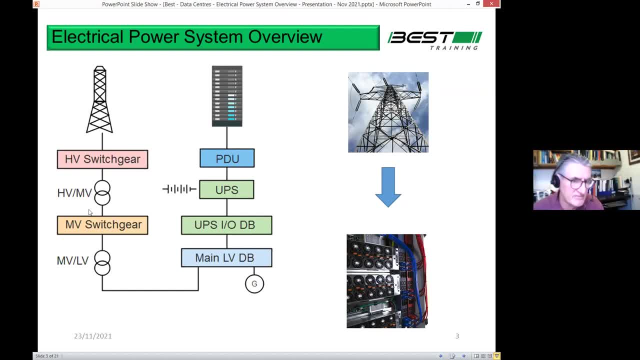 it covers our 10 kV system and our 20 kV system And it's either one of those two voltages you'd be distributing around the site. So then, when you get closer to the data centers, the buildings where the data is being processed, et cetera, you have to transform back down. obviously a safer. 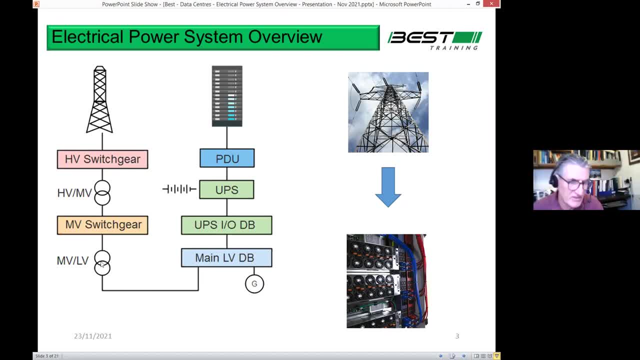 level of voltage, which is 400 volts, And we transform down to these MV LV transformers And you supply into a main board here. So the transformer is usually quite close to the main board, And then you have a generator feeding in. So you obviously 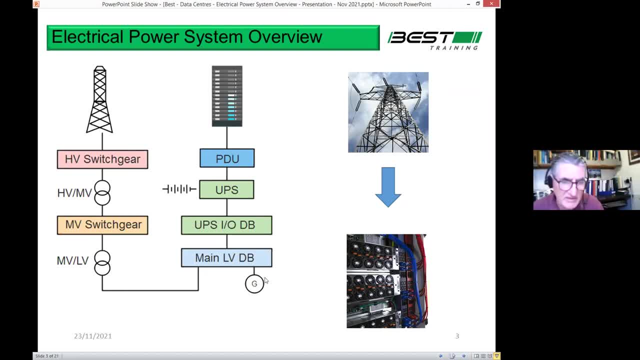 have to have a generator feeding in. So you have to have a generator feeding in, So you have to have a backup generator, because if the grid fails, the show has to keep going in the data center. It's processing all our data: our Facebook pages, WhatsApp messages and, of course, much more. 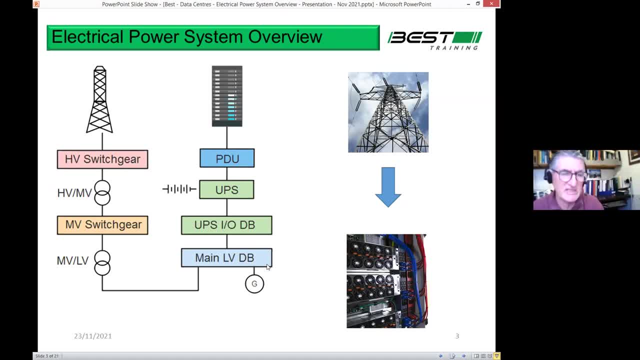 important things like banking transactions and all the other sorts of things that are running in the background, because everybody runs their business on the cloud now. So that's the diesel generator provides the kind of long-term backup if there's a long outage, But there's also a UPS. 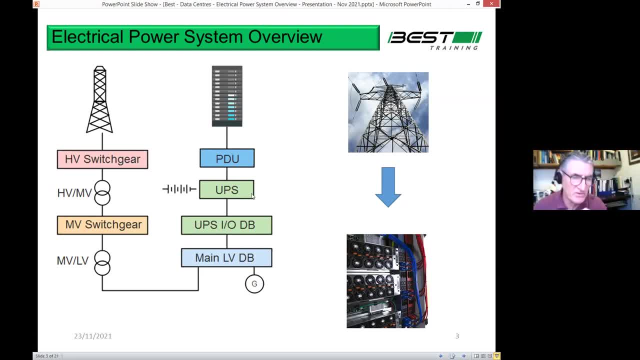 system. Now, the UPS is a battery backup system. It stands for uninterruptible power supply. It basically is a battery backup system that provides a no-break backup to the power system. So if the power fails, the UPS continues to deliver power without even a microsecond of a break. It. 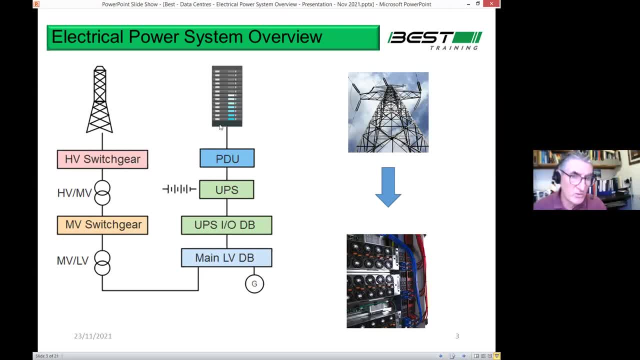 just continues to feed power to the essential load, which is, of course, the servers. And then the generator starts up And after about 10 minutes- sorry, about 15 seconds, I should say- the generator is online And it takes over and the UPS batteries start to recharge again. So this is what we're looking at. 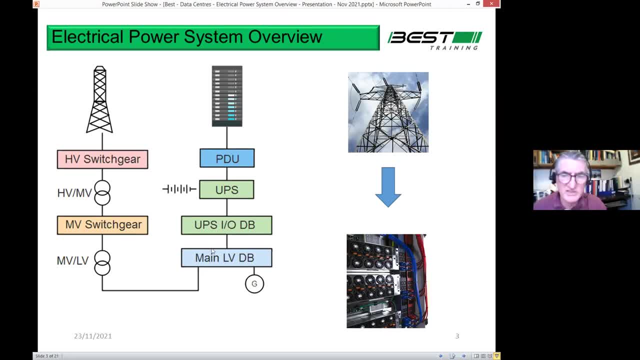 today- this with the main focus here- from the medium voltage switchgear down- And the right hand graphic is just showing it there- Big, big transmission pile in there, whatever that would be at 220 kV or 110 kV, And the power source is going right back into the back of the rack. This is the 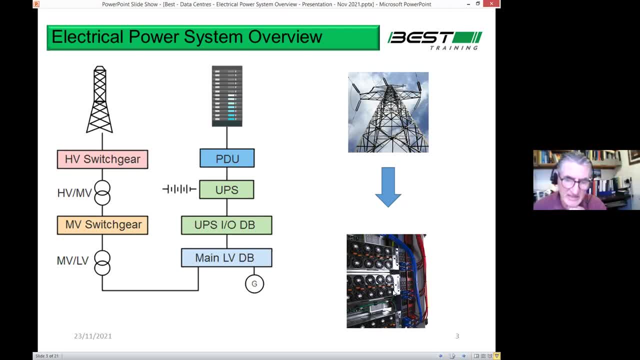 the servers, the back of the server rack, And you can see the power coming in here. the red and blue leads are the cables going up onto the actual server, And so we're going to talk you through all of that, Right, And the main components in the power system that we'd be looking at there. So, medium voltage. 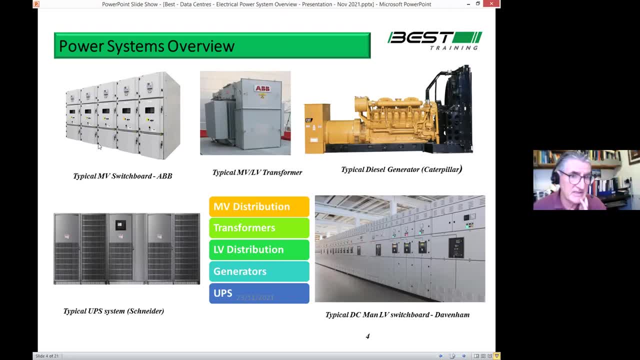 switchgear. that's what it looks like, So you can see there on the top left hand image there's, there's five cubicles, we call them, And each of those cubicles is a circuit breaker, So the equivalent of the little trip switch in your house, what you call it an MCB or the trip switch. 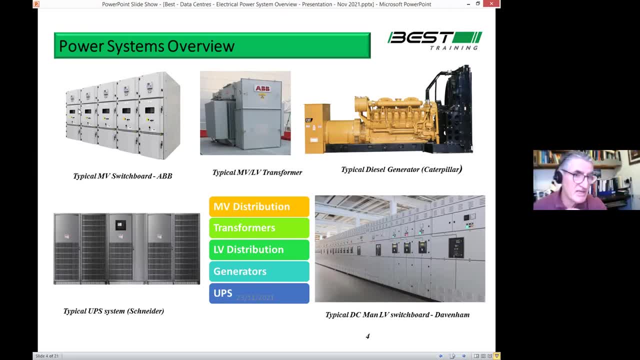 some people call it So that's what each of those are, But obviously they're handling vast amounts of power, So it's much more complex, much bigger, etc. Transformers which convert the power from high voltage down to lower voltage. That's what we're. 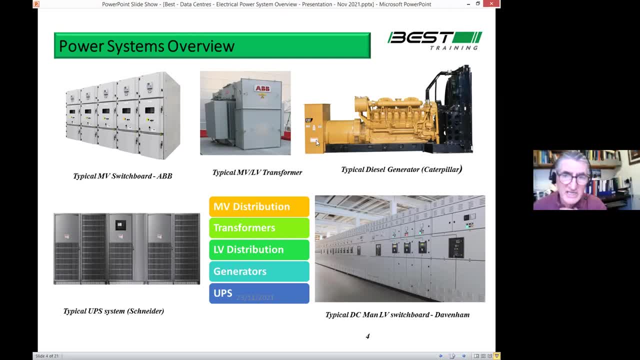 seeing there And we'll be looking at that- The generator, so the generators. that's the typical generator. there you can see the diesel engine is in the middle. it's just the same engine that you have in a big truck or anything like that, And radiator on the end of it and then it's driving. 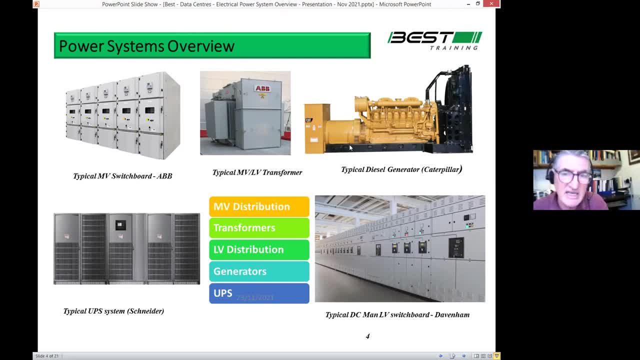 the alternator on the left hand side. The alternator is just literally a synchronous motor, if you like, and when it's powered by an external source and given some field current, it generates voltage, And that's the generator, And then the UPS system here is. this is what we call a static UPS system. 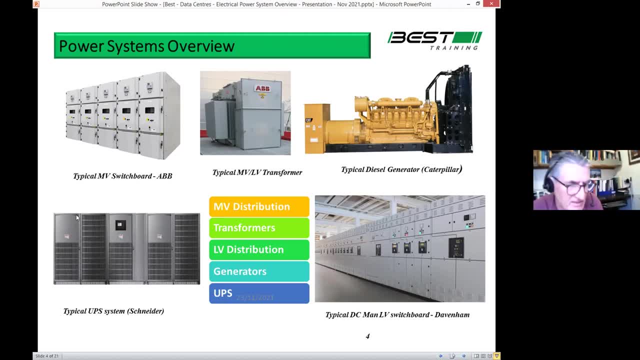 It's stationary, there's no moving parts other than the cooling fans in it. So it converts DC power to AC. So it takes battery power and converts it to AC and gives you a kind of a short term backup while the generator is starting up. And then the low voltage distribution system. So 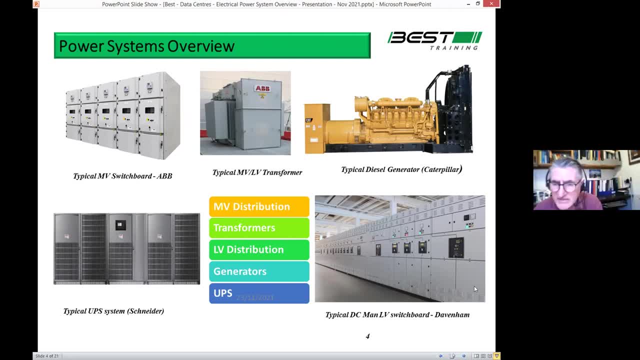 you can see that board. that's a typical data center board. You can see the length of that. that's probably 30 meters long, that board, And probably half a million quid's worth of switchgear in that. So that's the type of thing. 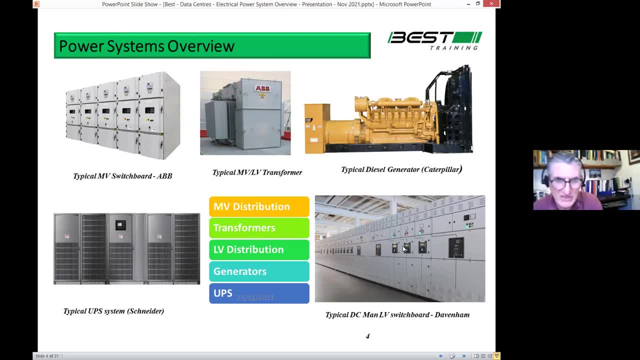 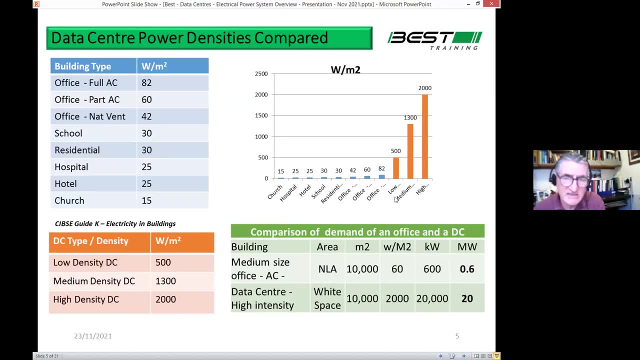 as someone quoted once to me, power data center does not come cheap. It certainly doesn't, So that's what we're going to be talking about anyway. So what's the big issue with data centers? again, a lot of bad news, a lot of bad press at the. 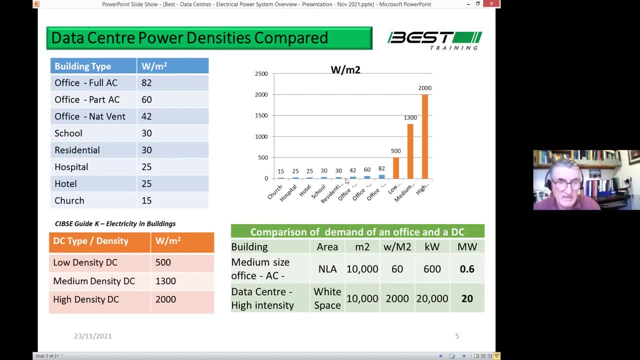 moment. Everyone's blamed them on our crisis on the grid or shortage of power and everything, And obviously they have contributed to it because they're close on, I think, one gigawatt of power heading that direction at the moment. So our maximum demand in the grid in Ireland. 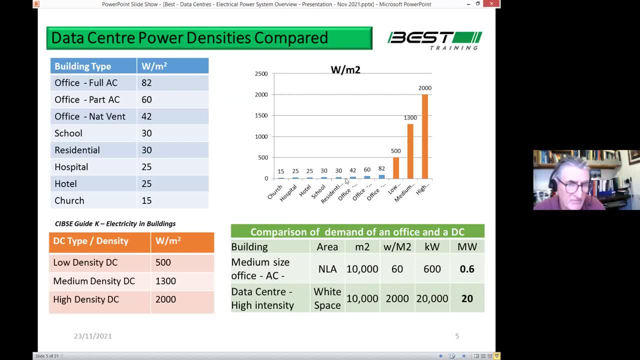 is about, say, five and a half gigawatts or something like that, And at the moment, approximately one gigawatt of our demand is due to data centers. So some people are saying that the problem I think they're really- are going to be part of the solution. 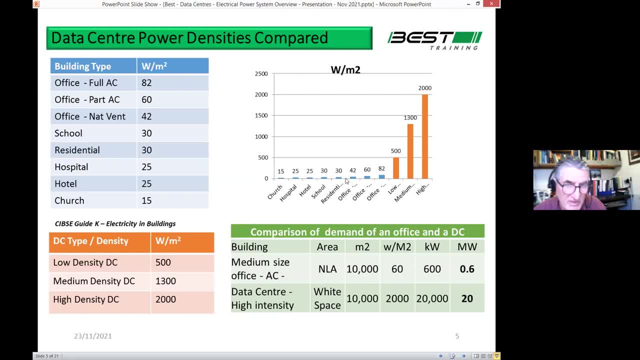 because the generators are going to be able, because they have an inherent backup power systems, they're able to come off the grid at a moment's notice, and that's the whole issue. that was in the Irish, the article in the Irish Times this morning. 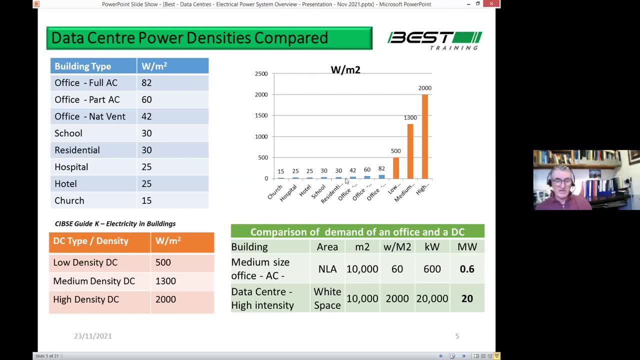 they're saying that data centers going forward, when they get their contract from air grid or ESB, whichever it is, it's going to stipulate that they must have their own emergency backup power system. So there's no surprise in that, because all data centers. 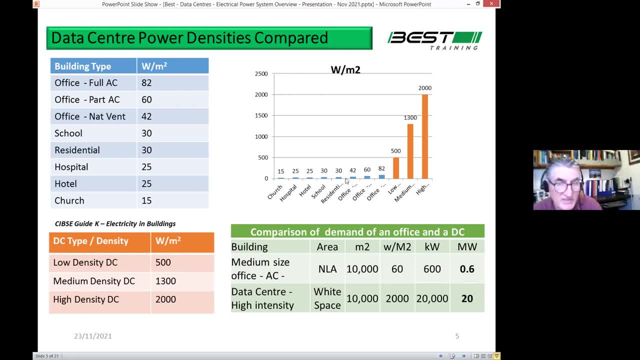 have emergency backup power systems. But the difference is now they're going to tell them you can have the power, but if we have a demand issue and there's an emergency power issue, we're going to have to take you offline and they're going to have to sign up to that agreement. 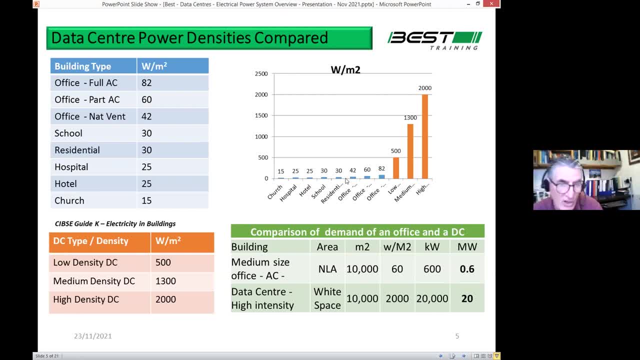 And I can see that being a problem, And I think they should be incentivizing even the older data centers that are here for a long time, incentivizing them to come off the grid at peak times and mitigate that risk that we're facing at the moment. 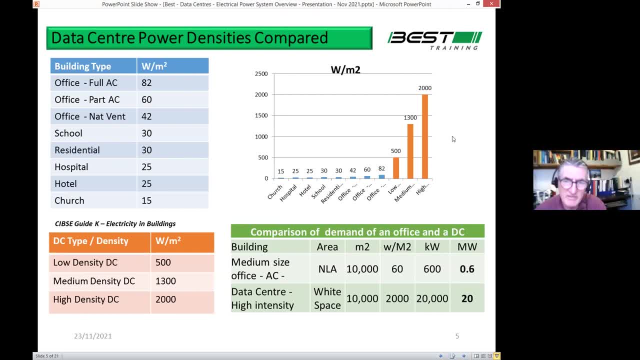 So what I've shown here just to explain what the whole issue is, the level of power that a data center takes. If you look in the blue table up here, the top left, it shows you different typical buildings, offices, schools. 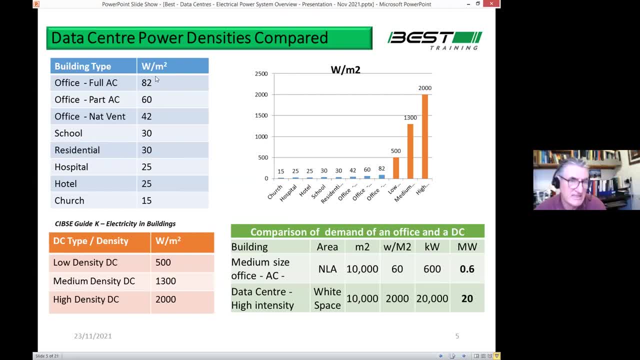 residential complexes, hospitals, And you can see their power. density is quoted usually in watts per square meter And what the square meter obviously refers to is the net lettable space on a school, you know the classroom space. It doesn't include plant room space or anything like that. 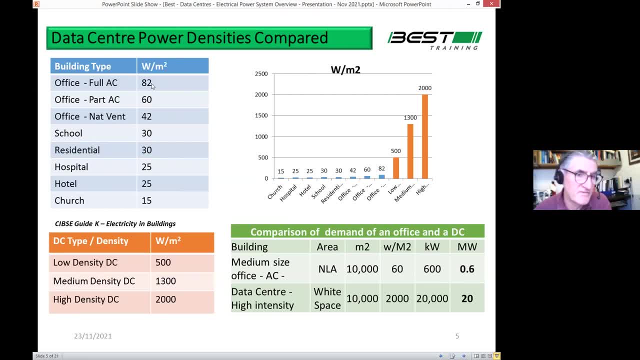 So it's the net lettable space of the building. So you can see, for a fully air conditioned office building it's quoted around 82. It'd be more typically around 60 now because air conditioning processes have changed and they've gone for natural ventilation a lot. 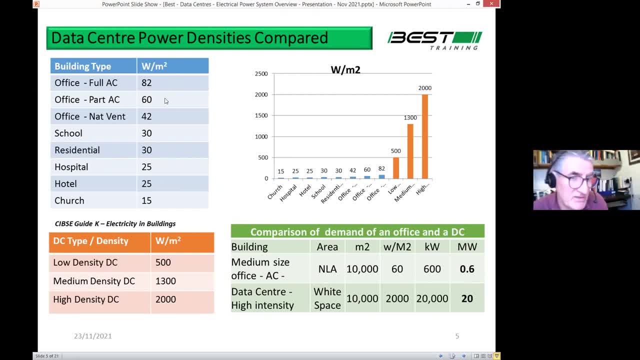 So a typical office might be taken 60 watts per square meter of demand down to something like hotel might be only 25, or a church or something like that bank, small building like that- 15 watts, You know there's hardly any load in it at all. 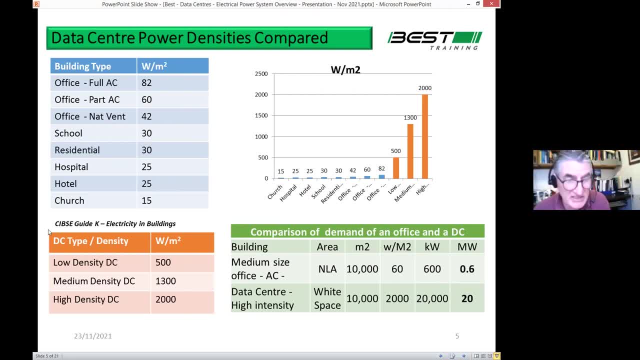 Now, if you look at that, I've just thrown those into a- sorry, the data center once. then I've shown down the end: low, medium and high density: 500 watts per square meter or up to 2,300 watts per square meter. So that's the data center. once then I've shown down the end: low, medium and high density: 500 watts per square meter, or up to 2,300 watts per square meter, or up to 2,300 watts per square meter, or up to 2,300 watts per square meter. So that's the data center. once then I've shown down the end: low, medium and high density: 500 watts per square meter or up to 2,300 watts per square meter or up to 2,300 watts per square meter. 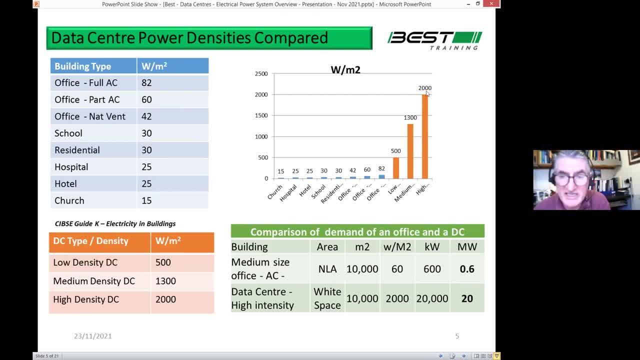 If you throw that into the graph, you can see the difference. So a high intensity data center is 2,000 kilowatts. That's two megawatts, a big part. two kilowatts per square meter, not two megawatts. 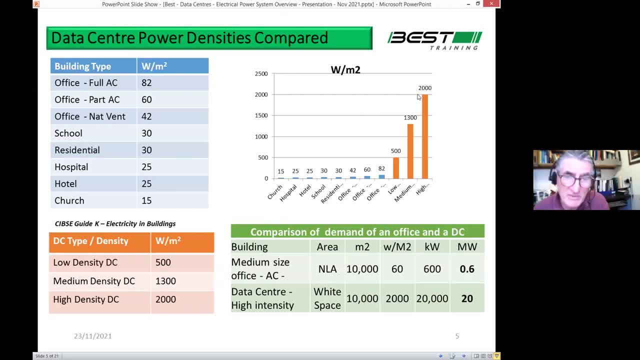 two kilowatts per square meter. To put that in perspective. if you can, we can all imagine an electric heater. you can see them in Power City or wherever. Harvey Norman, you know what it's like plug in an electric heater. 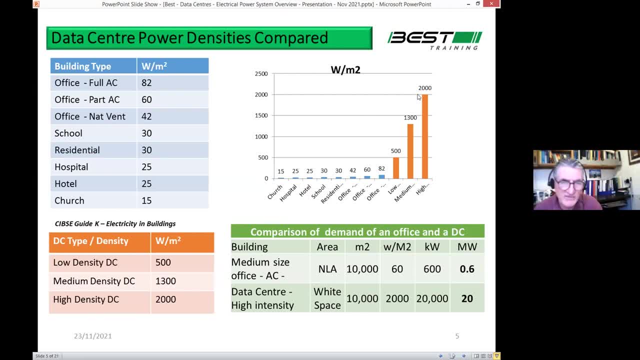 and you can feel the heat of it. Imagine just having 20 of them in the one rack and then thousands of racks in the one building. That's what you're facing. So that's how you end up with. typical data center has thousands of kilowatts. 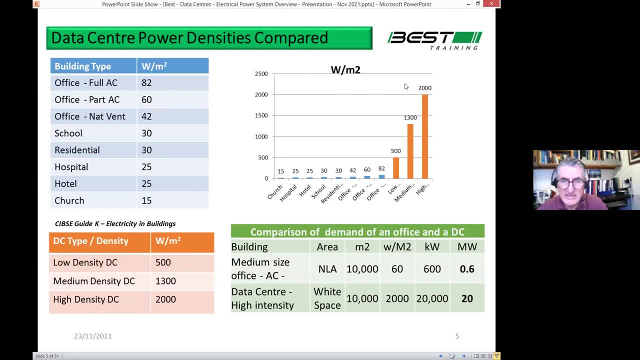 which we call megawatts, of course. So I've done a little comparison down here: different buildings, So a medium-sized office. okay, We're in a net nettable area of 10,000 square meters, So it only includes the office space. 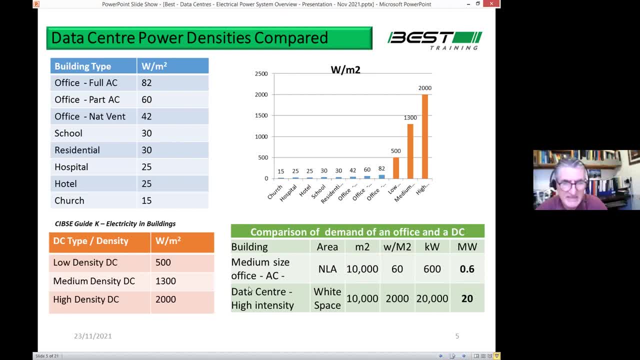 the circulation routes, et cetera. It doesn't include the plant rooms And the data center that we're looking at. then we're looking at the white space. So in a data center, the white space means the area where the data is actually processed. 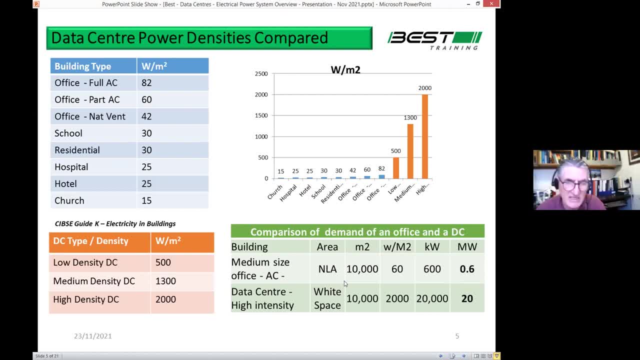 It's like the production line in the factory. It's where all the racks and the servers are, So it doesn't include the electrical plant rooms and the ventilation plant rooms, et cetera. So two of them compare them. like what like. 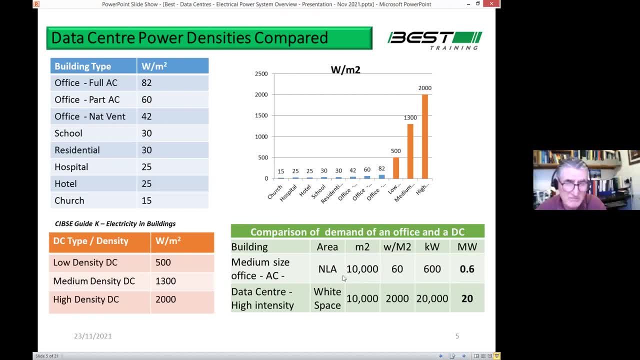 10,000 square meters in each case. So 10,000 square meters will be a medium-sized office, like one of the offices you see along the north wall, there in the office. you know banking headquarters, that type of thing. 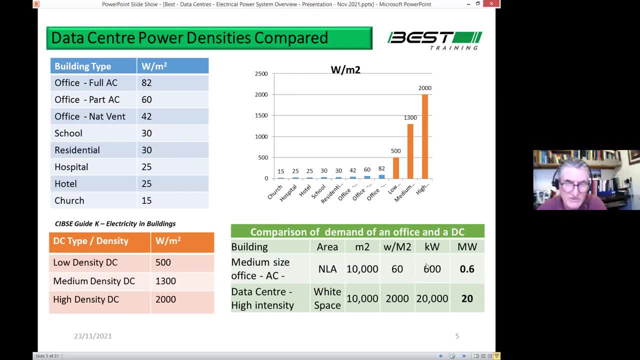 10,000 square meters, 60 watts per second. 60 watts per square meters gives you 600 kilowatts, or 0.6 megawatts, to get the language right. So we're talking megawatts, right: 0.6.. 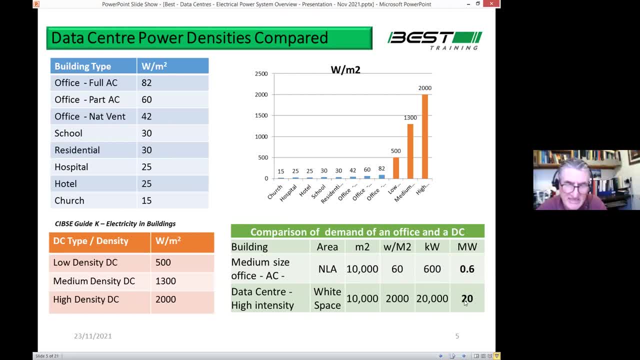 The same flow print for a high intensity data center is 20 megawatts And that's typically what we're talking with with data centers- 20 megawatts. So you can't just connect 20 megawatts on it. 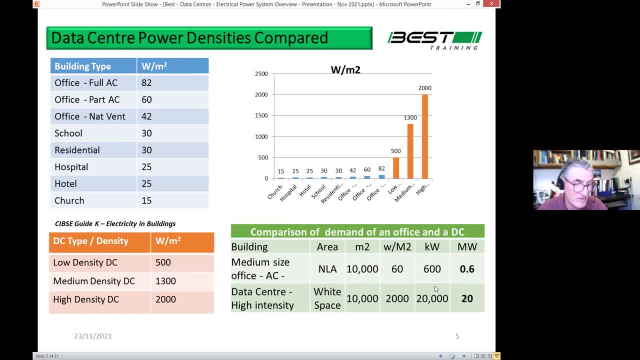 get onto the ESB and say: listen, I'm building a data center, Can you give me 20 megawatts? And they make a connection under the pathway. That doesn't work like that When you get to 20 megawatts. 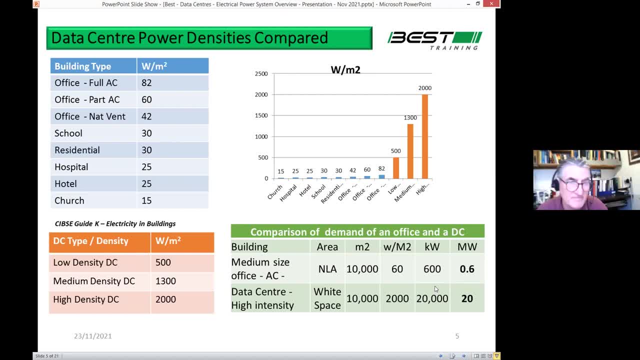 you have to take power directly off the transmission grid. So that's the big difference. Whereas anything at 0.6 megawatts you're coming off the medium voltage network. 20 megawatts you're at transmission level, So you're connecting at 110 kV or 20 kV. 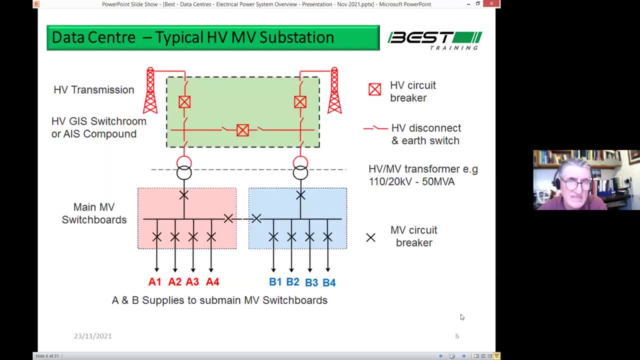 110 or 220 kV, sorry. So that's what we're talking about. So the typical data center. an overview now. these are very simplified schematics, obviously, and there's only so much you can show in a PowerPoint presentation. 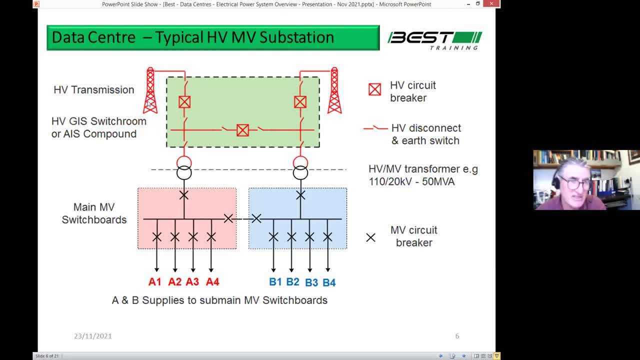 But you can see what happens here. You have the pylons here, So this is either 110 kV or 220 kV network And they literally break into the line and bring it into a new. they build a new substation dedicated to the data center. 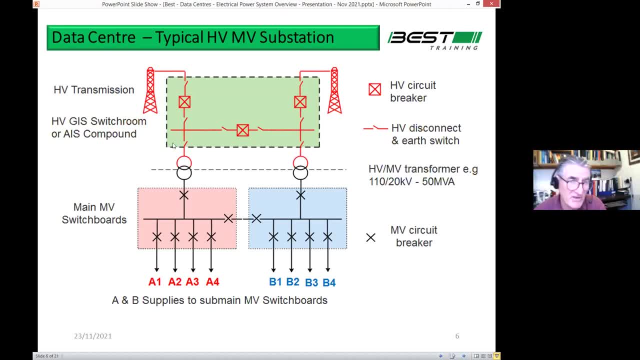 Now, when I say they, the data center operator obviously pays for all of this and very often develops the substation themselves- what's shown in the green box? but it's the ownership of the ESB. So what you're seeing inside the green box. 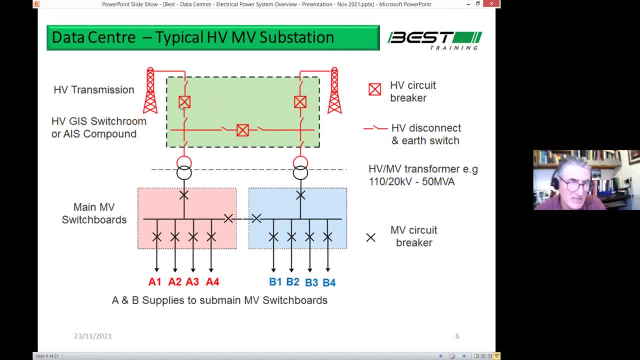 is connection of. one pylon comes down through a circuit breaker, that's the box with the X in it, And the other switches then are called what they call disconnects- high voltage disconnects, to be able to isolate the circuit breaker. 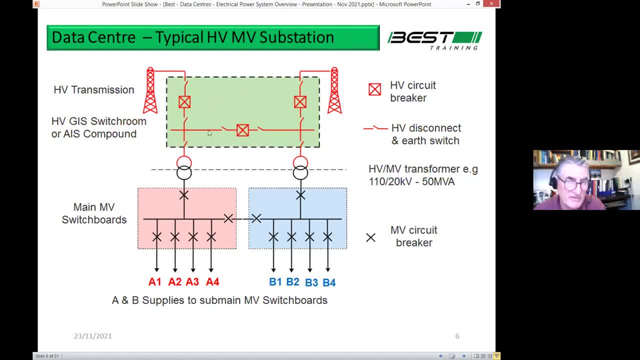 So the circuit breaker on each side and then both supplies then are coupled through this arrangement here. So it gives the ESB flexibility to do different switching operations. So again, as I say, that's not normally part of the building services consultant's job. 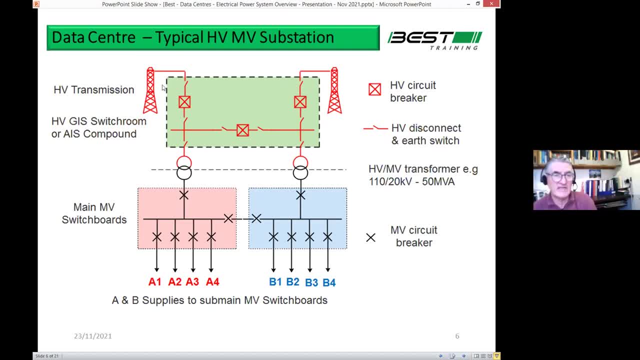 And certainly I've never gotten involved in anything that level. I'm just showing it at a very simplified level at this stage. So the building service consultant normally starts here on the medium voltage side. So you have the transformers here converting power or transforming power down from 220 KV. 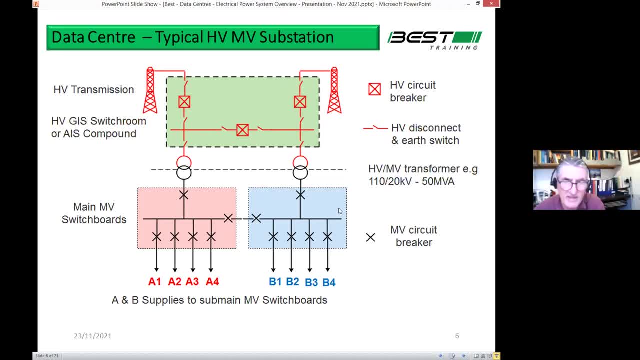 or 110 KV down to 20 KV, So those transformers are typically 50 megawatts. It's typically, you might say, 50 megawatts of power each day handle, which is enormous. You notice the size of a large town. 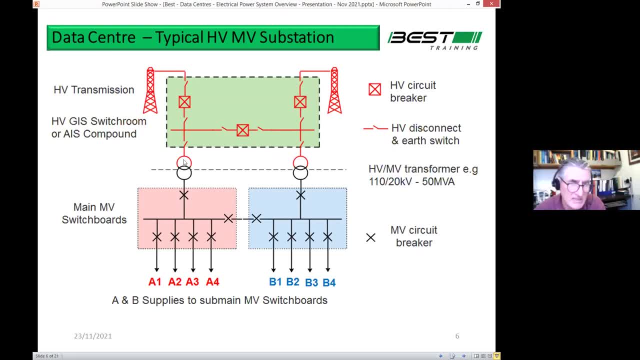 will be taking that sort of power And then the supply comes out at medium voltage and you come into an A board and a B board And we're going to explain a little bit about resilience and redundancy. Everything is duplicated in data centers. If the A system fails, you have a B system to back up. 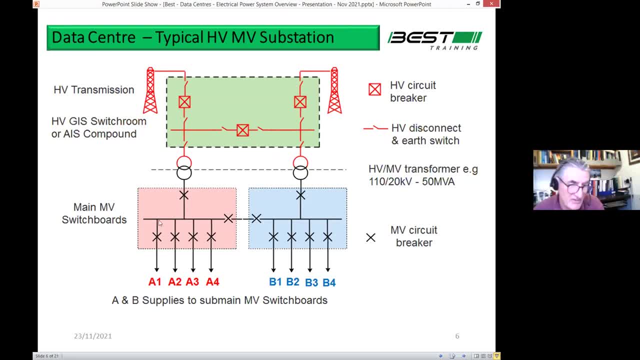 And it's typically done like this: You have an input circuit breaker, then you have a number of feeders going out, feeding out to your other transformers around the site, And the two boards are coupled together here. So if you want to take one of the transformers out of service, 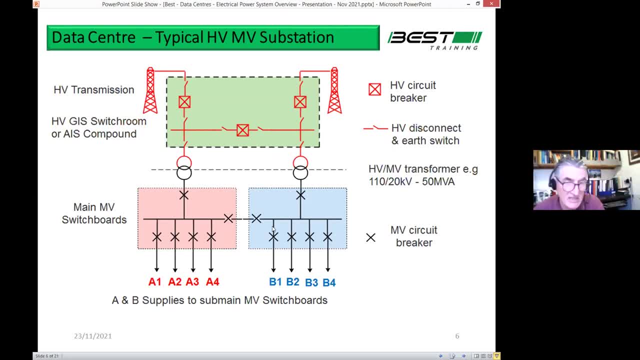 you can join the two boards together, et cetera, and lots of different configurations. So that's the basic high level overview Of the power system And we're going to look at these various components. keep drilling down all the way to the back of the rack. 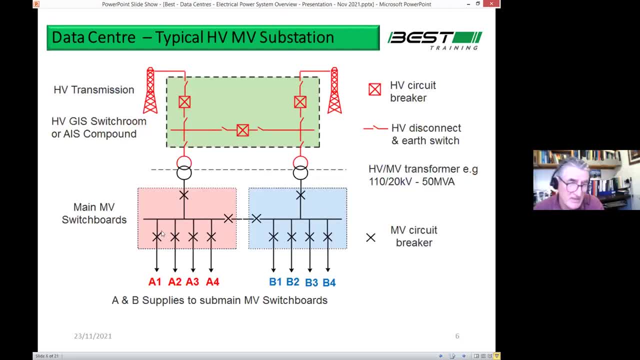 So if you see this diagram I'm just showing as an example, there's four supplies on the A side and then four supplies in the B side. So in the next diagram you're going to pick those up and what happens with them. 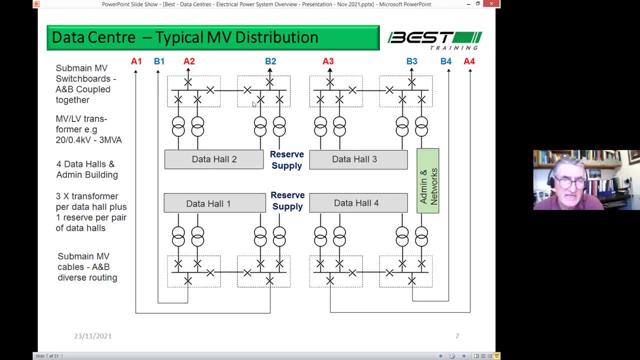 So you can see there's A1, B1, A2, B2,, et cetera. So this is just one. there's multiple ways of doing it, configuring the power system, but this will be fairly typical. This is showing. 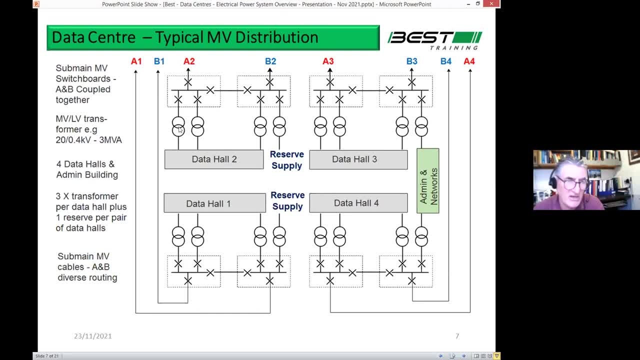 this is a data center with four data halls and each data hall has three transformers feed And you can see there, just say, data hall two there on the top has three transformers feeding into it And each of those transformers are typically something around three MVA, three megawatts. 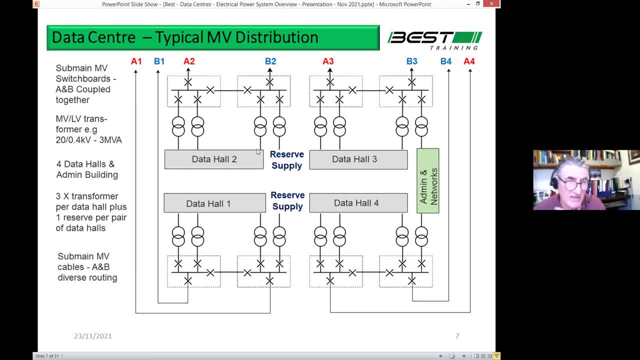 So that means there's nine megawatts of power going into that data hall And all that's in it is racks, racks after rack after rack, just full of servers processing all our data and storing our data and processing it in our, as I say, our watch. 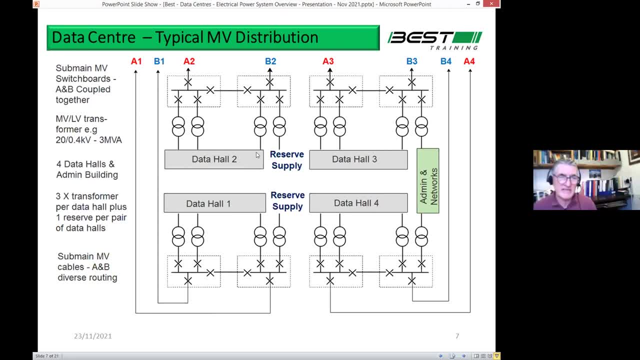 our WhatsApp messages, our Netflix movies, our bank accounts, everything we do, smart vehicles going forward, smart cities- all that's what they're all there for: the processing all that data and saving it, storing it on, et cetera. 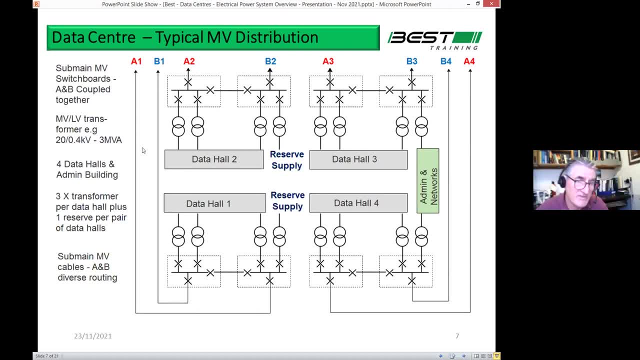 So in this case you have three transformers, So there's about nine megawatts of capacity going in there, but the servers don't use all the power. So nine megawatts- if nine megawatts is going in, there's approximately probably around six to seven megawatts. 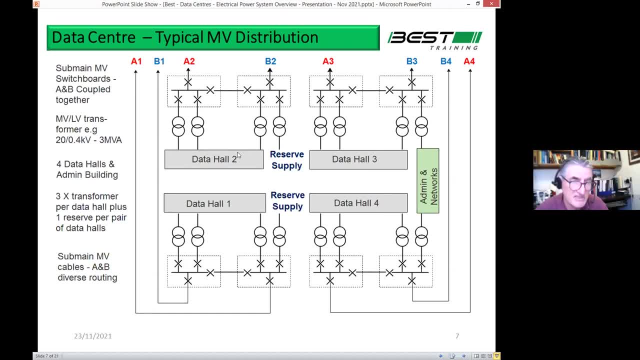 would be used for processing. So nine megawatts would be used for processing data And the remainder of the power is used to cool the plant, to cool down the service, And there's different ways of doing that. We're not going to talk about that today. 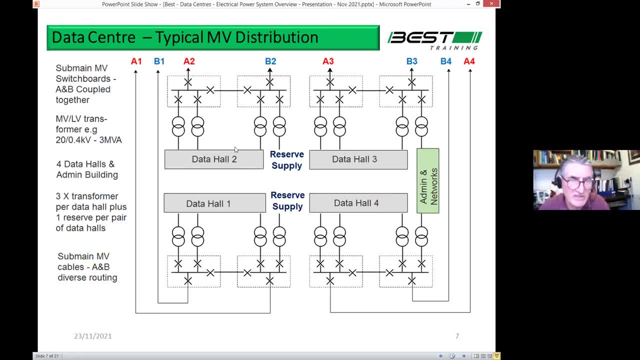 but you can have air cooling, chilled water, refrigerant cool. There's all different ways of doing it- Like obviously cover that in the main course that the data center course will do. So each of the data halls have three transformers, So they're kind of really a mirror image of one another. 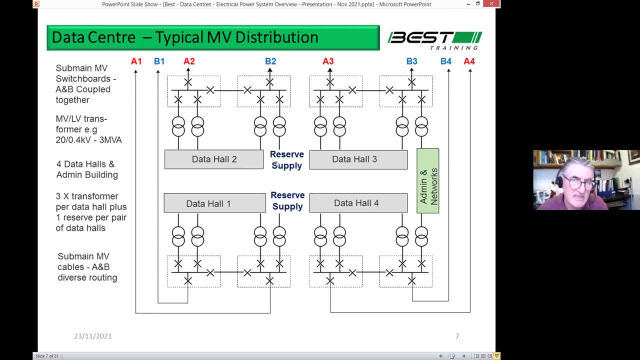 And then you see there's a reserve supply in the middle. So the reserve supply is like your plus one, your spare system that you have here, And that spare system then can take the place of any of the other transformers to the left or the right. 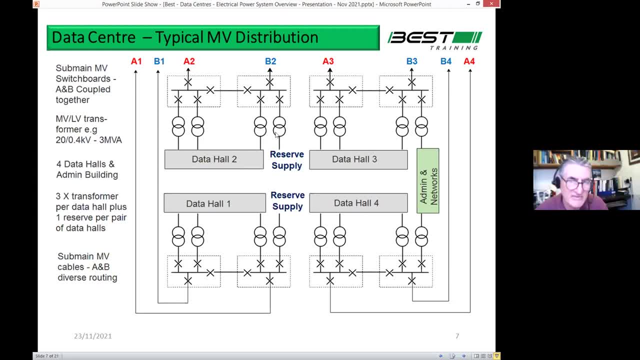 So if one of the transformers has to come out of service, this reserve supply can be switched in. I haven't shown it on the schematic how it's switched in. We look at that later. It'd be too complex to show on this diagram. 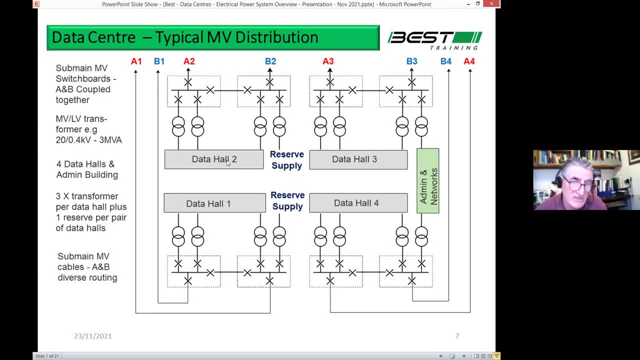 And then the other thing you have in a data hall. of course it's not just all about servers. The servers have to connect to the outside world And that's why most all data centers have network rooms where the outside fibers come in and they go in. 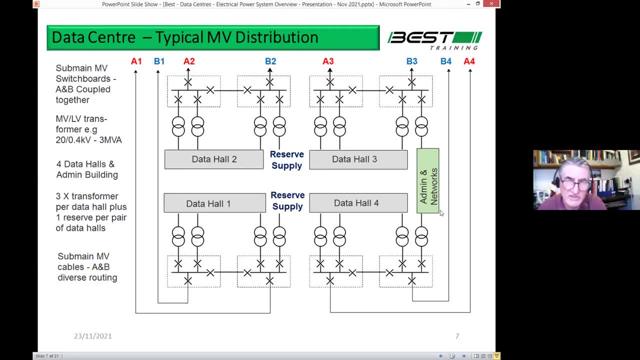 and link to all the various data halls And that's run through the network buildings And, of course, you have admin. then you have meeting rooms, toilets, offices, canteen- all the normal things you have in every other building in a data center as well. 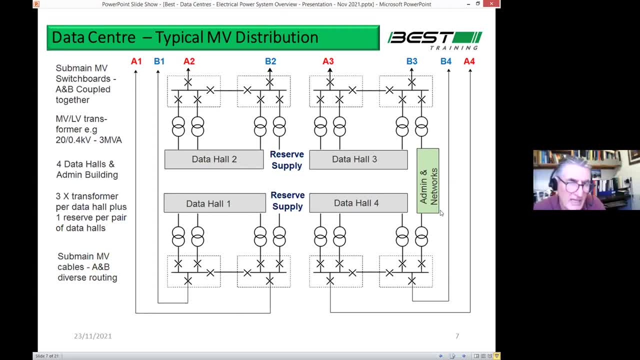 because they're not all just unmanned. Most of them have a permanent staff in them, a small amount of staff in them, and they have to have all their normal other building functions. So let's look at some of the stuff then that appears. 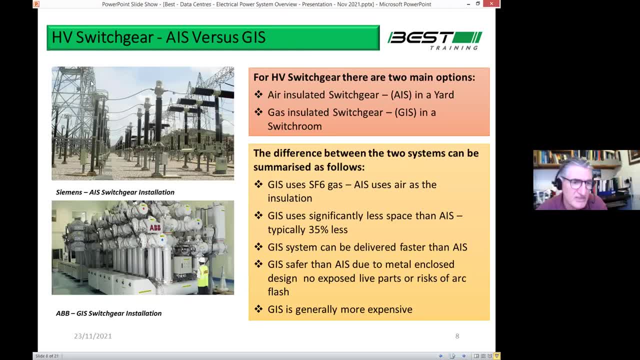 So when we looked at the high voltage connection, first of all there's two options. you can see the top image here. That's what we call air insulated switchgear, And it's called air insulated switchgear because, literally, the conductors are insulated. 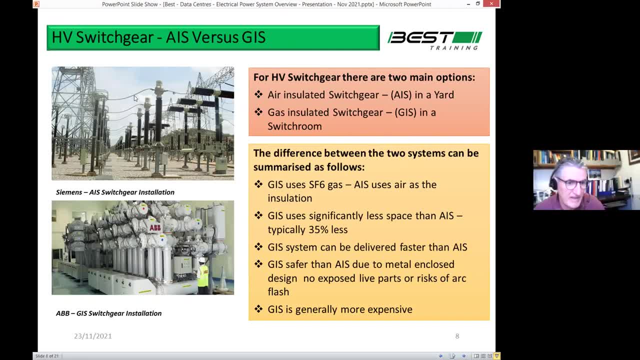 from one another by air. They're typically separated by the phase one, from phase two to phase three, et cetera. It's separated in air, typically maybe one and a half, two meters apart, as you see there. So the power comes in and the pylons drops down. 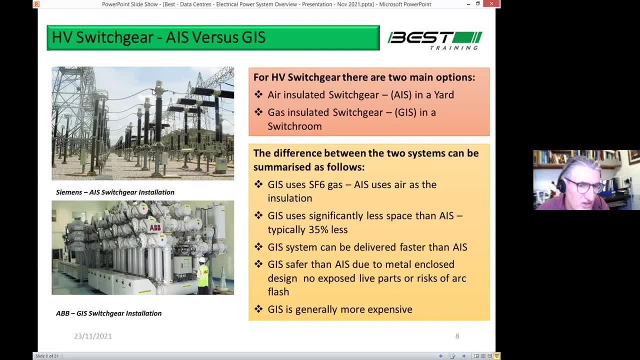 and you can see all these insulators et cetera And these are things like current transformers, circuit breakers, disconnect switches and things like that. So it takes up a vast amount of space this type of switch gear arrangement. 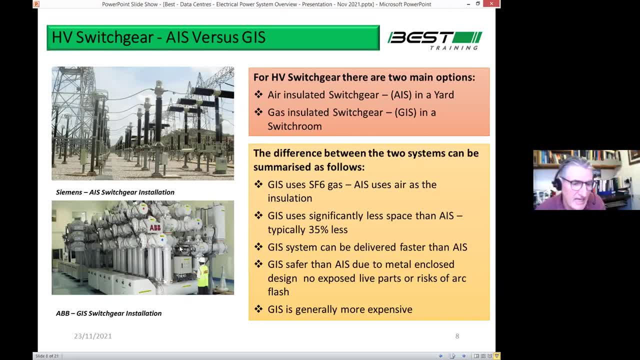 So that's what we call air insulator. It's called AIS for short. And then gas insulated is the same thing. We're dealing with high voltage, but instead of insulating by air, the conductors are all contained in these enclosures. 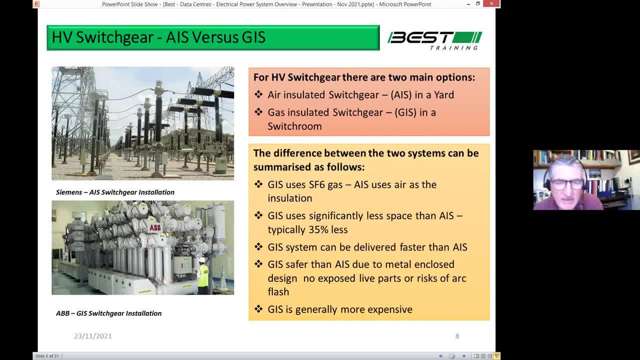 which are filled with SF6 gas, which, of course, has a bad name from an environmental point of view. If it leaks. it is it has. it has a very, very high negative impact on the environment in terms of global warming and ozone depletion. 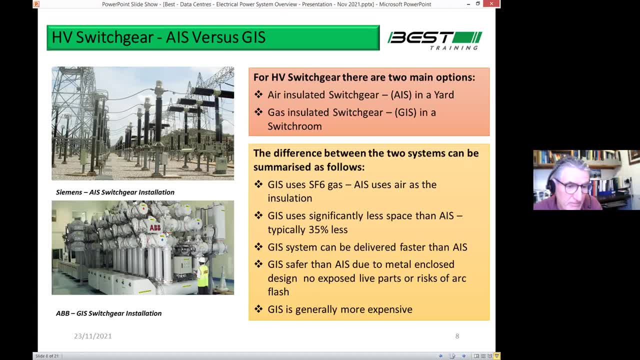 and all those things, And so for that reason it has to be very carefully monitored. But the advantage with the gas insulated is it's extremely compact- probably somewhere around one third the space that an air insulated switch gear installation will take up. So again, this is usually built by the data center operator. 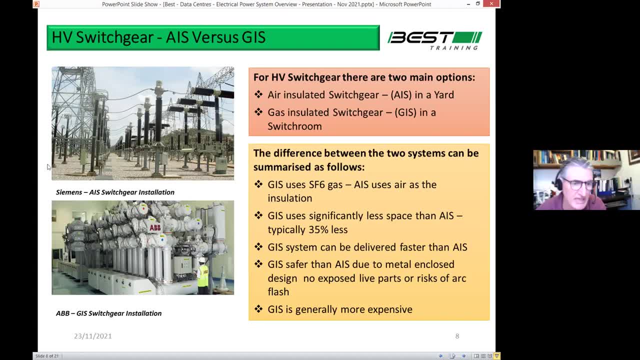 in Facebook and Clonny, which probably a lot of people know about. It's out there just to give you an idea that I worked on the first phase of that, which was three buildings And the first connection was 120 megawatts. 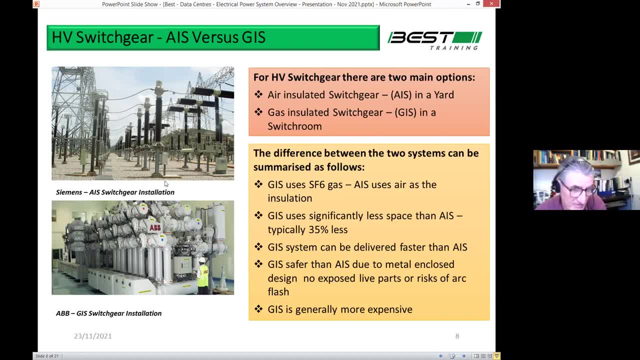 That was for phases one, two and three. They're now on phase. they're building phase five, I think, or phase six, if I'm not mistaken. So, and that's they have a massive big air insulated switch yard like that. 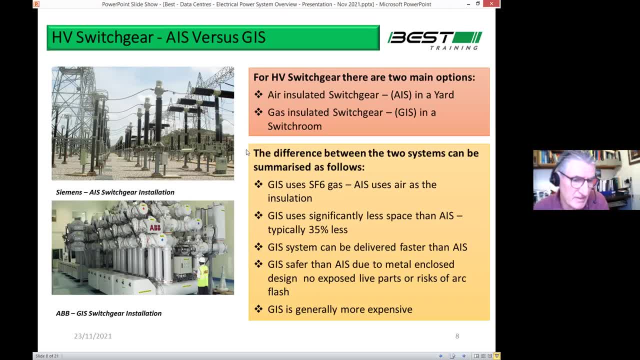 And you know at this stage they probably have 200 megawatts of capacity on the site. So it's just phenomenal. And smaller data centers might go for this air insulated switch gear arrangement, but in either case it's built by the data center operator. 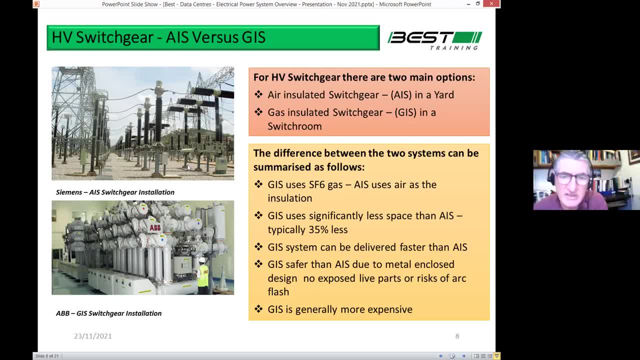 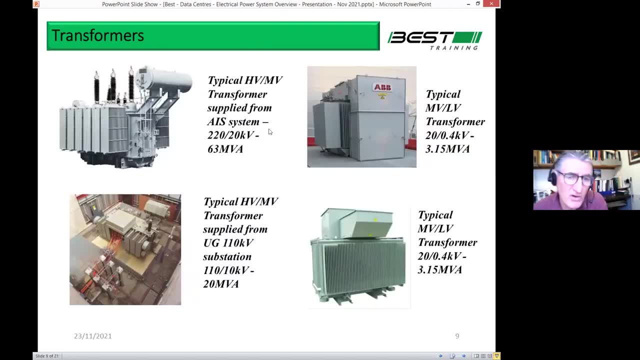 and then handed back to air grid as opposed to the ESB. So that's really the two options. when it comes to the high voltage side, Then transforming down, I'm showing two different- well, four different- types of transformer here, And the top one is where you transform. 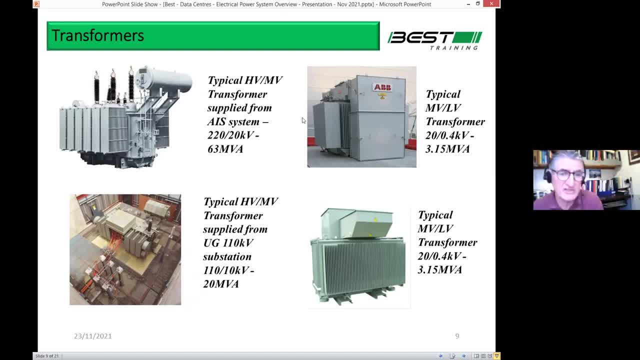 from the high voltage down to medium voltage. So high voltage, just to remind you, is either there's either 220 KV or 110.. There's also 38 KV on our system And it's rare. I don't think there's any data centers connected to 38.. 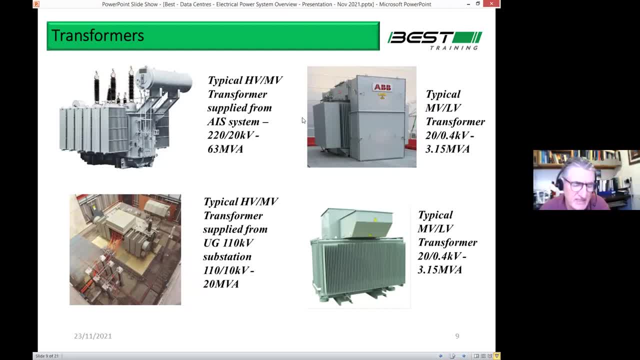 I think most of them are connected at either 110 and the data center- Facebook data center- is 220 KV. So that's what you have there. Typically that would be as part of an air insulated switch gear arrangement. You can see the bushings on the transformer here. 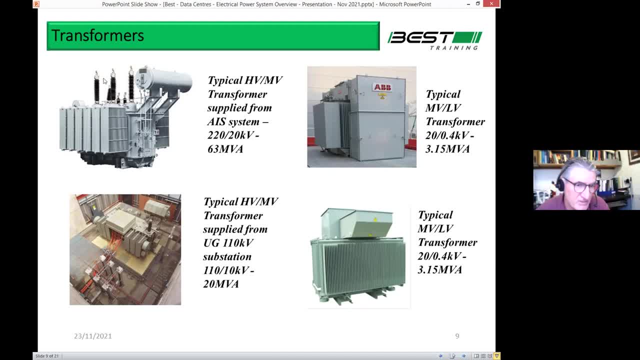 So the taller ones are the higher voltage. So it comes in here at 220,000 volts- 220,000. Just think of that- Thousand times higher than the voltage in your house. And then it goes outside at 20 KV. 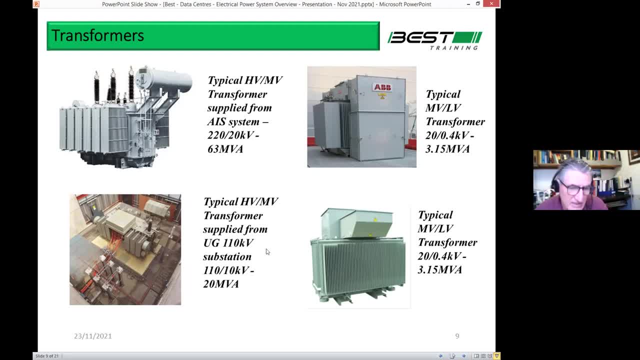 The one down below then is another data center I worked on. This is out in Clonshock And this is 110 KV down to 10 KV, So it's a smaller transformer. This one is 20 megawatts, The one above it is 63 megawatts. 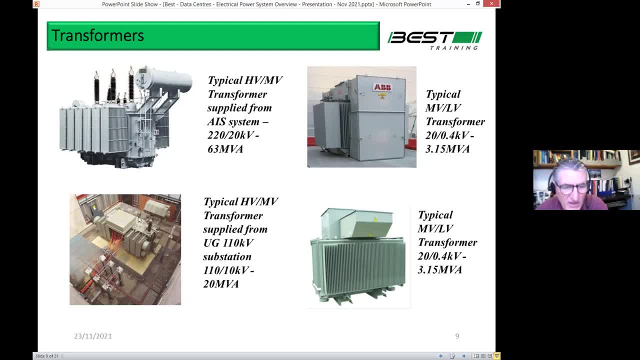 So that's a typical one that's fed from an underground supply from the ESB, a remote ESB substation. So it's kind of different arrangement. So they're HV to MV transformers. The two on the right then are MV to LV. 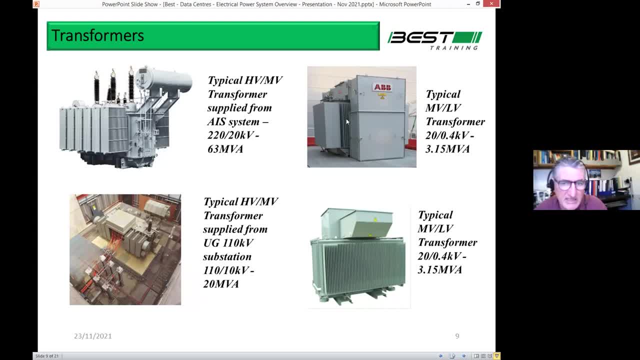 So transforming from 20 KV or 10 KV down to 400 volts, So 400 volts, 400, 230 is the standard voltage we use in commercial, industrial buildings et cetera In your house, as you know, it's 230 volts single phase. 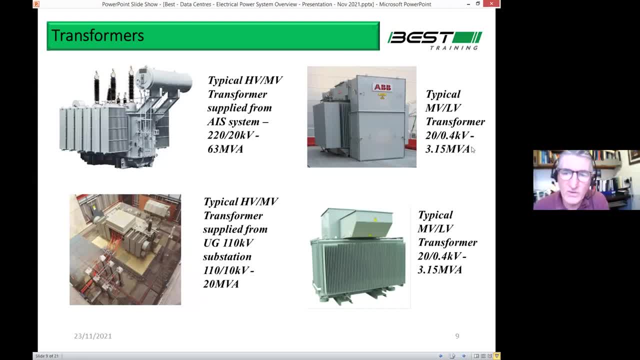 but in industrial and commercial buildings they use three phase and it's 400, 230.. So that's for these transformers: transform it down to the final safe voltage that you can distribute it around the building et cetera. And the top one is typically about three megawatts capacity. 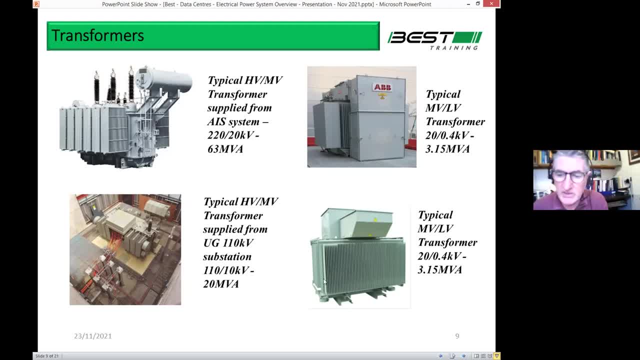 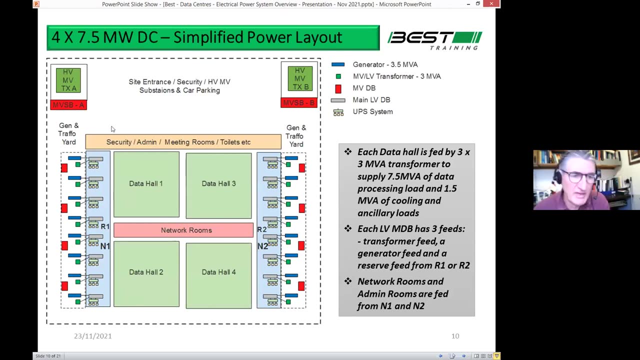 And the one down the bottom is it says three megawatts. That's a copy and paste error. It should be about probably about one megawatt or 1.6 MVA, whatever So so translating that into a simple floor plan. 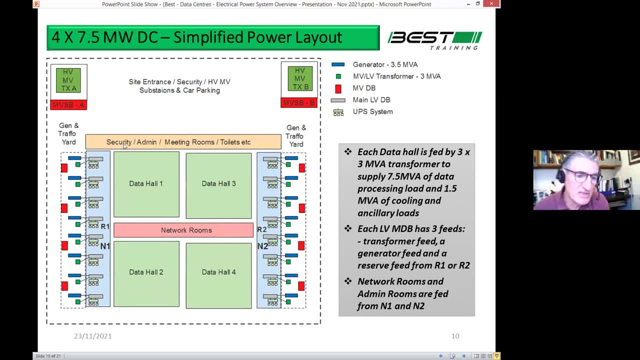 what it actually looks like. It looks like in the data center. So again I'm showing data center with four data halls. I literally made this up out of my head. It doesn't represent any particular data center. You probably will never see a data center like this. 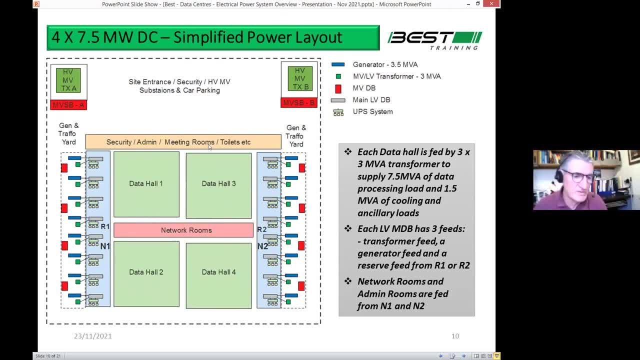 but to explain how all the where all the different equipment goes, I just use as a simple little block diagram. So the outer dashed line here represents the perimeter fence of the data center. So when you arrive up to this place you can't just throw your leg over the fence. 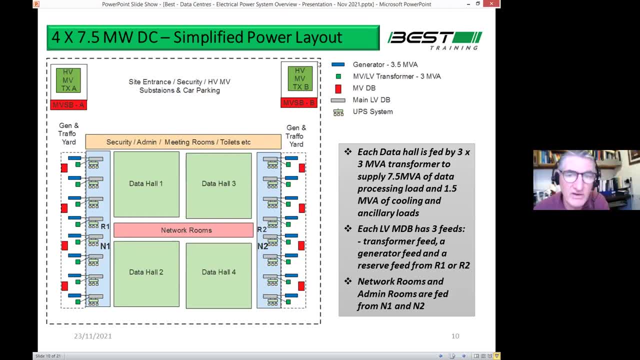 and walk up to the data center. They're highly, highly secure environments, for obvious reasons, So they're usually have a very high protective fence around the perimeter And then, as you come in, you see the four green boxes in the center. they represent the data halls. 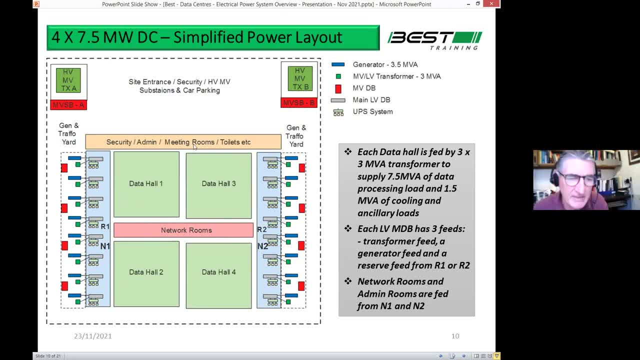 and the kind of cream color at the top, security, admin, meeting rooms et cetera. And then on the outer side, then you'll see there's kind of two blue boxes. They're what they call the electrical plant rooms. 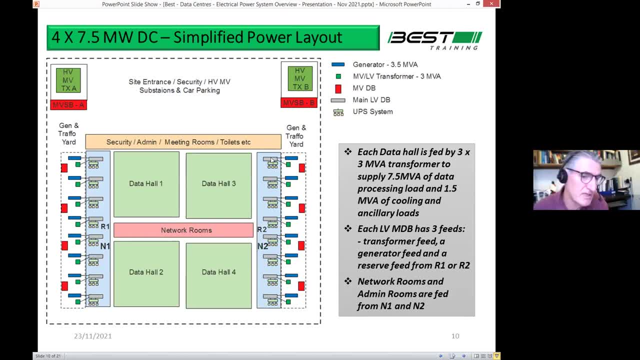 Now I'm not showing any cooling here, where the cooling plant room, because the cooling could be on the roof or it could. you know, you could have a different configuration. The cooling could be around the perimeter of the building or it could be on the roof. 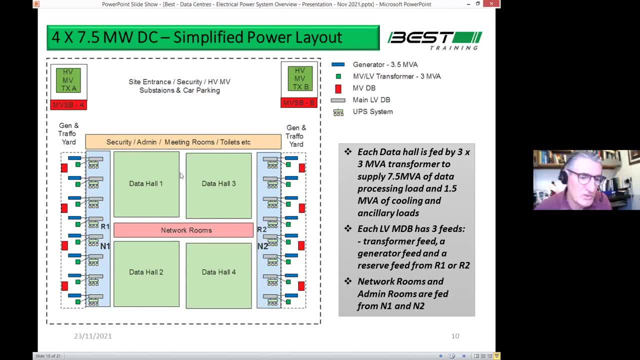 So we're not getting into that today. This is just a notional schematic showing where everything would go. So what we're going to look at is first of all the top left-hand corner and top right-hand corner. you see HVMV. 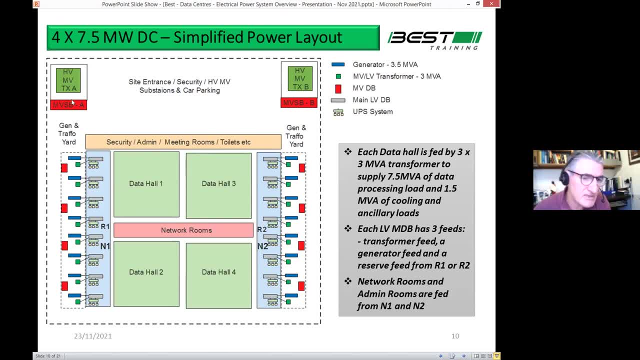 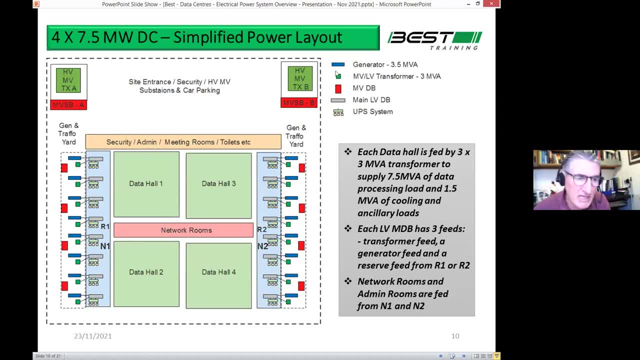 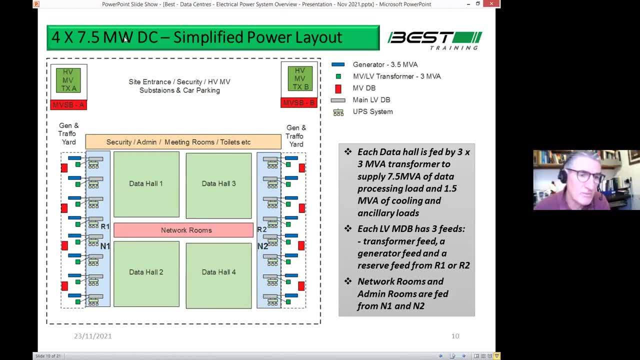 in case the proverbial bomb hit one, it wouldn't damage the other, et cetera. And then somewhere else, which I haven't shown the schematic, you have the ESB HV substation, This substation that brings the supply in from the pylons. 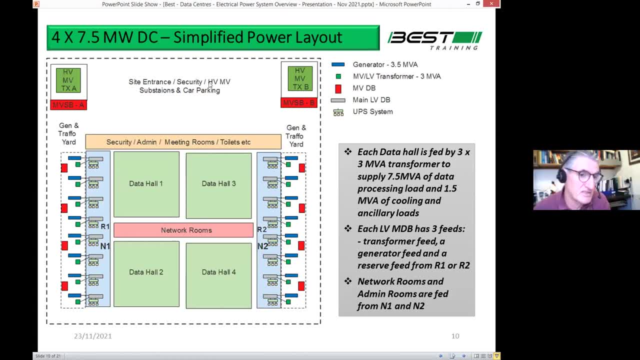 And it's not shown in the diagram here because it could be anywhere. It could be any configuration. Some of the sites, the substation is actually remote. The ESB bring cables from their substation into the site. So that's what I'm showing here. 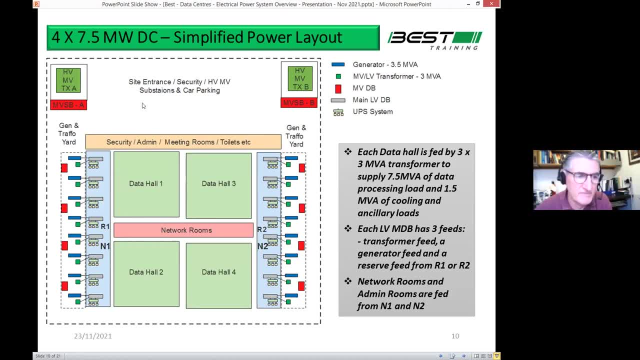 See if the two transformers, the A transformer and the B transformer, transform from HV to MV. And then you have your MV switchboard shown in red. You have your A board and your B board. You'll start getting a feel for it very shortly. 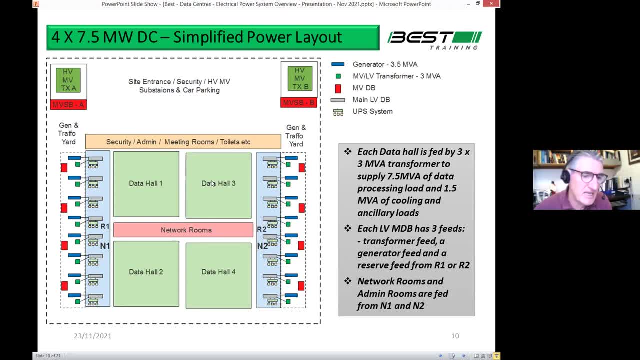 Everything is duplicated or has a spare reserve system backup. So what we're going to look at now is a typical data hall. I'm going to take data hall one, for example, and look at what switchgear is associated with that, So you can see to the left of data hall one. 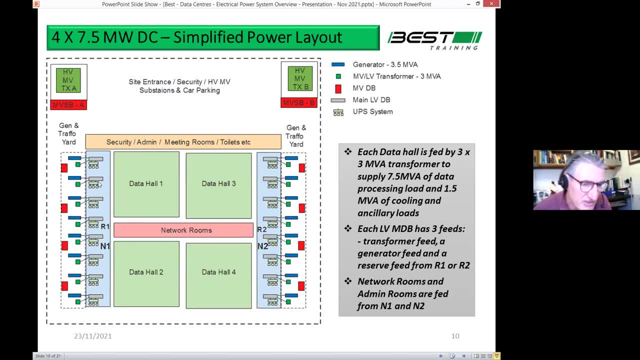 you have three gray boxes, followed by three green boxes, et cetera, And what they represent is: the gray box represents the main LV switchboard And if you look out from the main LV switchboard you'll see it's fed with a generator. 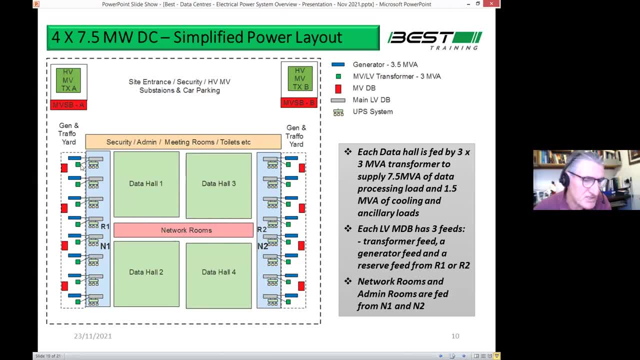 and the little green box beside it represents the medium voltage to low voltage transformer. So the medium voltage low voltage transformer has to be right beside the main board, Very, very close, because the cables coming off it are absolutely massive. So you try to keep that as close as possible. 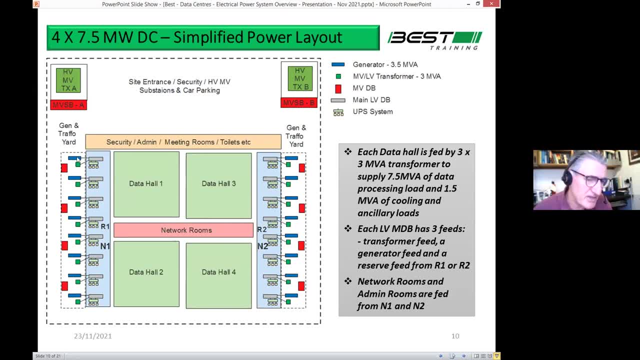 to the switchboard, And likewise with the generator, The red box. outside then is the MV switchgear which feeds the transformers. These green boxes are supplied at 20 kV typically from the red switchboard here, And that module just repeats itself all the way around. 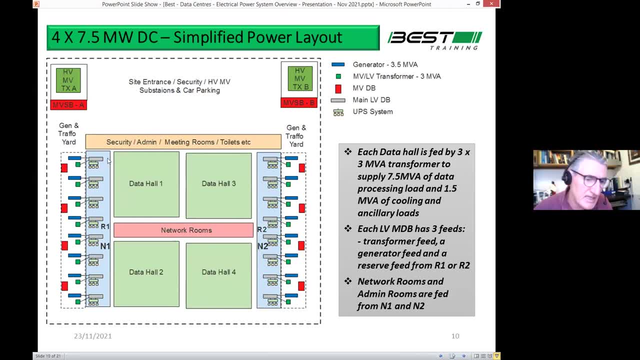 So in this case, if you want, the basic building block is about a three MVA transformer and a three MVA generator feeding into a board, And that board then in turn feeds down into the UPS system And the UPS system then in turn feeds power directly. 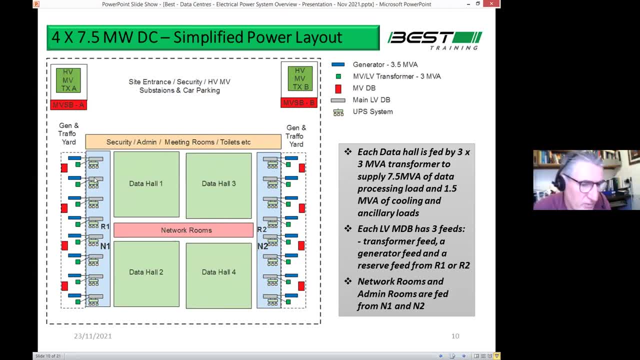 to the server? Well, not directly. There's a whole series of other equipment that feeds through before it gets to the servers, But that's where the servers draw the power from. So the other stuff that would be fed from the board, we haven't shown it here. 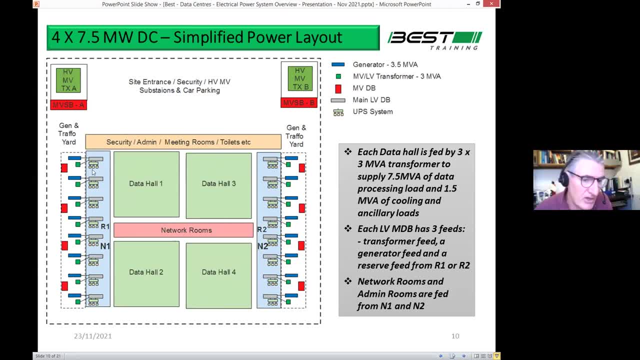 is the cooling plant and things like lighting, small power, all of those other things that a building needs to function, But our focus today is on the server, So that's all I'm really showing here in it, So you can see that. 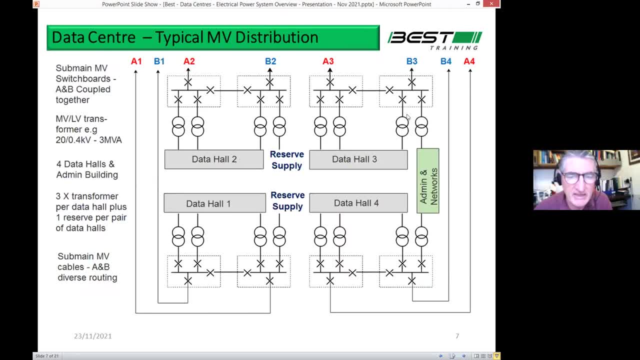 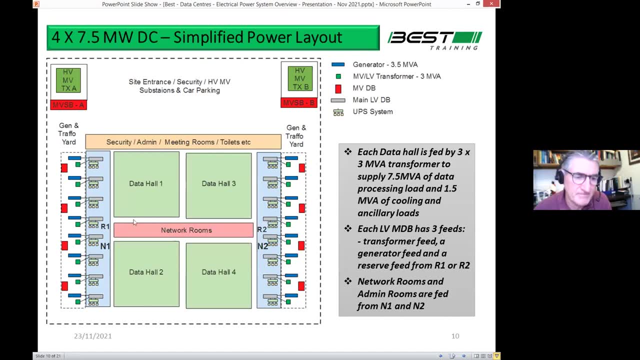 that really is a schematic representation of what we a plan version of that schematic. really, That's what I was trying to create, that in plan form, Four data halls and each data hall has three transformers, three generators, And then in the middle you have a reserve. 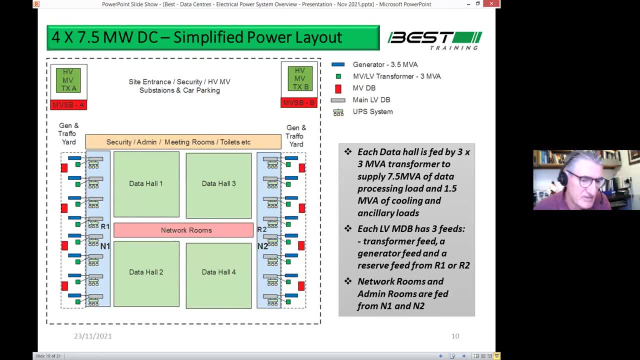 So if any one of these transformers or generator fails, the system is designed so they can pick up power, they can take power off the reserve system here And we look at that in a few slides, I think. Ah, next one. I didn't realize it was coming up so quickly. 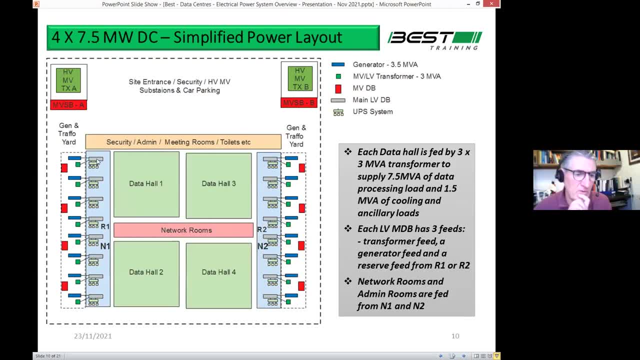 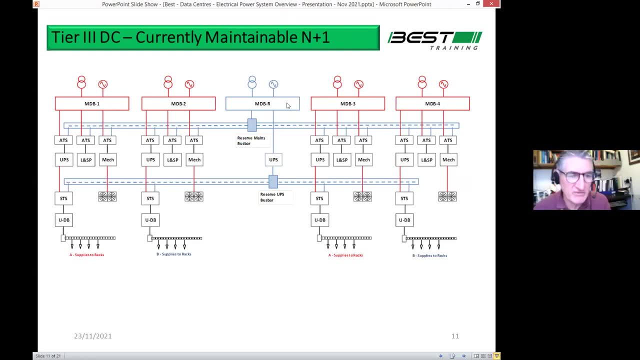 Okay, So in this case I'm showing three boards here, then a reserve, then another three boards. In the schematic. I'm only showing two boards and a reserve, just for simplicity, As I say if I put the six in. 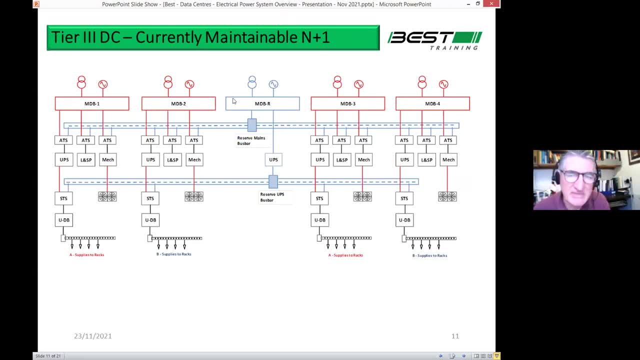 you wouldn't be able to read the diagram. So this is typically what happens schematically now. We're down at the medium voltage level now and getting in from medium voltage down to low voltage. So we're down a good bit down through the power system. 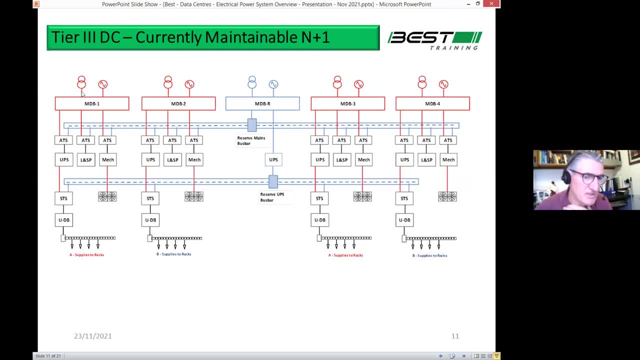 at this stage. So you have your transformer convert medium voltage to low voltage. You have your generators feeding into the board. Now, if we look what happens in each board, each board feeds down and feeds through this thing called an ATS. I'll explain about that in a minute. 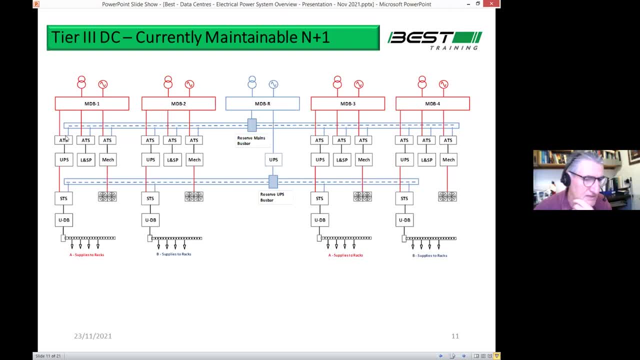 It stands for automatic transfer switch, but the power comes through that and then feeds the UPS system which feeds the servers. L and SP stands for lighting and small power. So all the lighting in the building, small power, small fans and things like that. 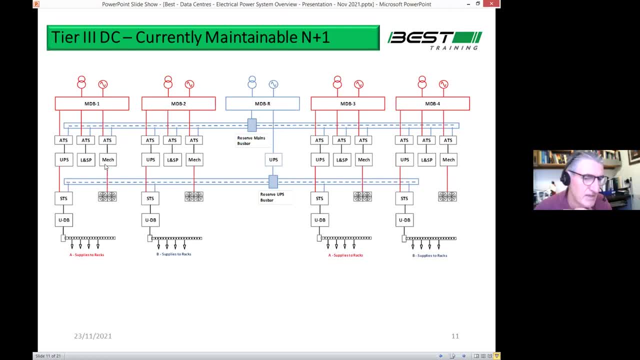 And then the MEC. it refers to MEC cooling system. So there are the three main loads. really. you have fed off each board in each data hall: UPS, lighting and small power and the cooling system, whatever that is, chill water fans, whatever it is. 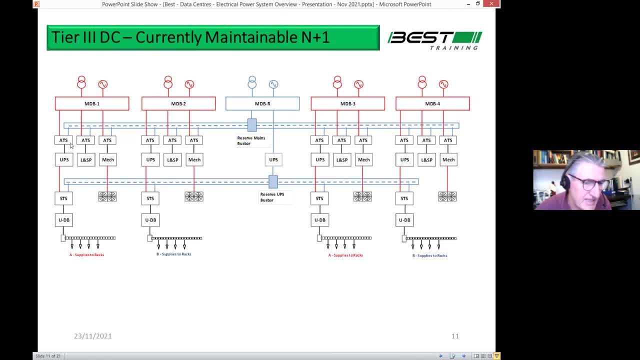 Now you'll see. each of those three loads is fed through the ATS that I referred to. ATS just stands for automatic transfer switch, And an automatic transfer switch just allows you to transfer the power from one source of power to another. Now, in this case, the red is the primary power. 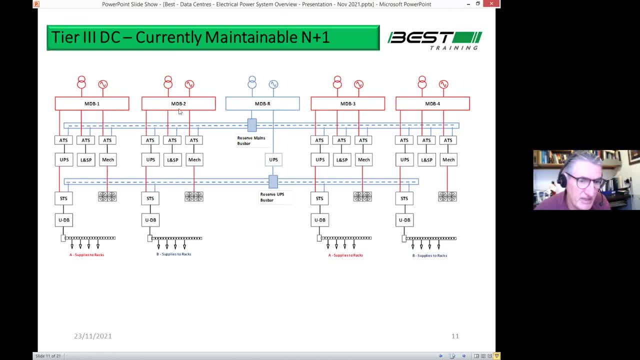 coming off the main board. okay, So you can see. the next system has a red board as well And the blue is the reserve. So the blue comes off the reserve system here and it allows it means if you want to come in and plan. 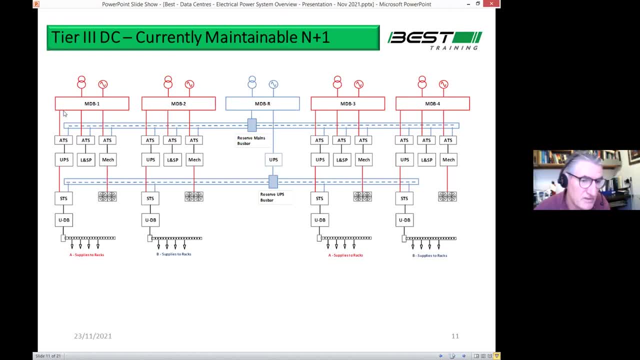 say, I want to take this main board out of service and work on it. well, I don't own my servers off that board to sit down, So what you do is you transfer the power over onto the reserve line And then you work on MDB1, you service it. 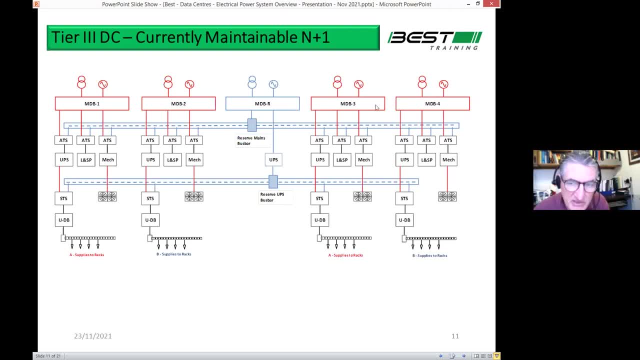 Then you work on MDB2 a month later and you service it on MDB3 and 4,, et cetera. And of course, it also works in the event of a fault. If the system power failed, the first thing it would do is try and start its generator. 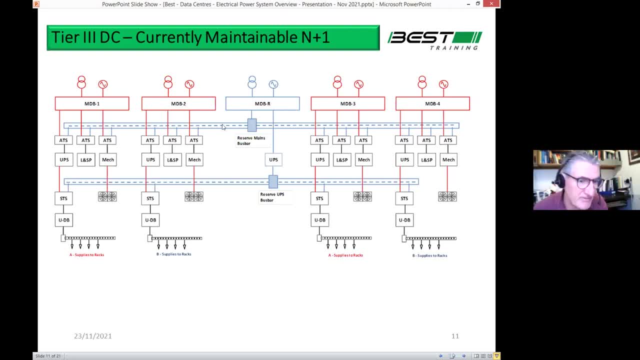 If the generator didn't work, then well then it would transfer onto the reserve line. okay, Now, when we get further down, you will see you come through the UPS. So the UPS which we'll talk about in a few minutes. 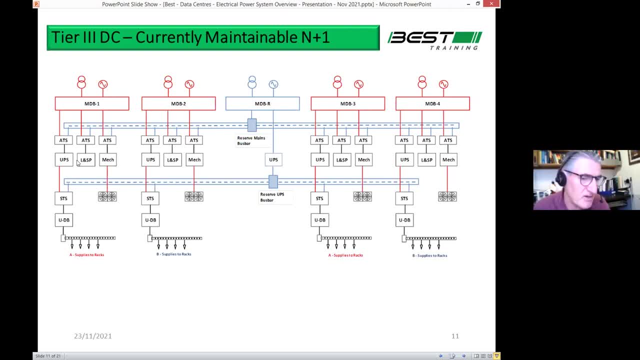 the UPS is your battery backup system that converts battery power into AC power And it's a no-break supply arrangement And that provides power down to your UPS distribution boards and out to the load. So you see, I'm showing A supplies to the rack. 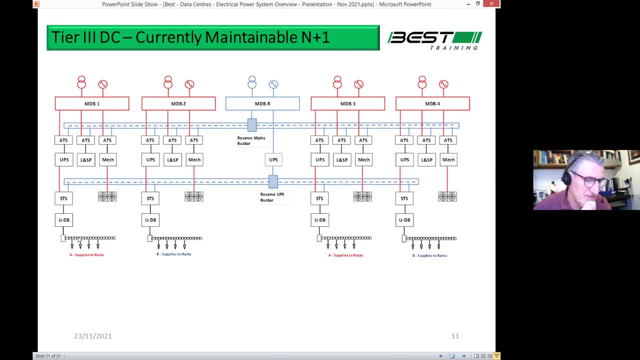 then B supplies to the rack typically. So it means that every rack has an A supply going into it and a B supply, And then every server connects to an A and a B supply. So you're bringing that resilience all the way down from the right, from the HV network right down to the back. 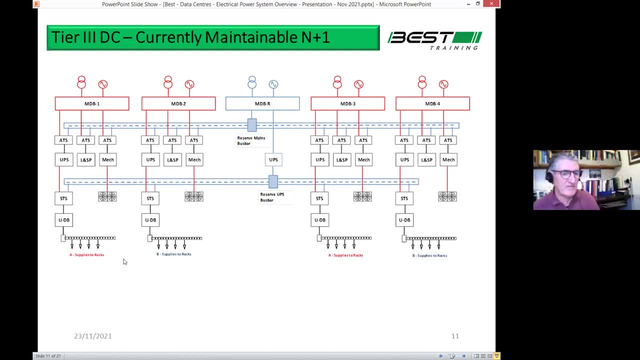 To the back of the rack. that is a dual pathway to every single server. If one supply fails in pickup it automatically picks up the supply off the other one. But to make that work on the UPS we end up having to have a reserve UPS distribution system. 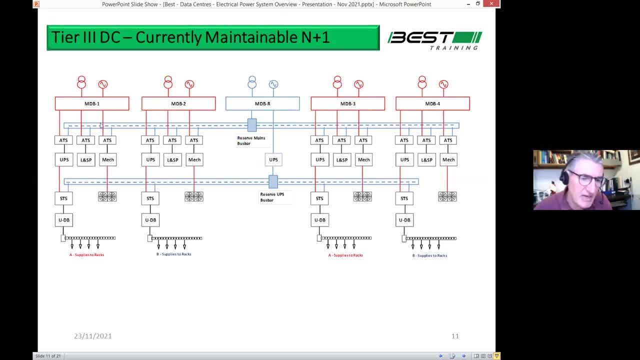 as well. So the top blue line there represents the power distribution system for mains power And the bottom blue one coming down this way represents the UPS reserve power system. And you'll see now they go through a similar switch, but in this case it's not an ATS. 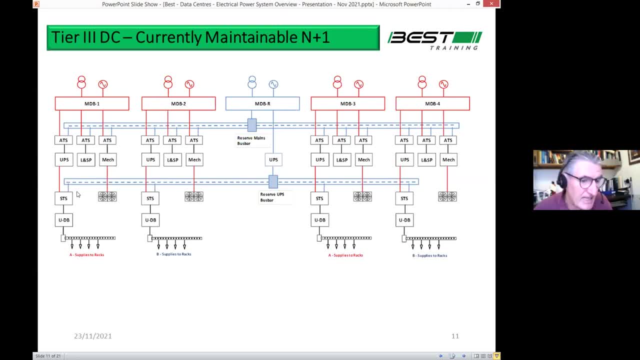 it's called an STS, which means static transfer switch, So it's static. It changes over to an electronic transfer system which the transfer from one to the other is in the order of milliseconds, maybe a very three or four milliseconds. the transfer is. 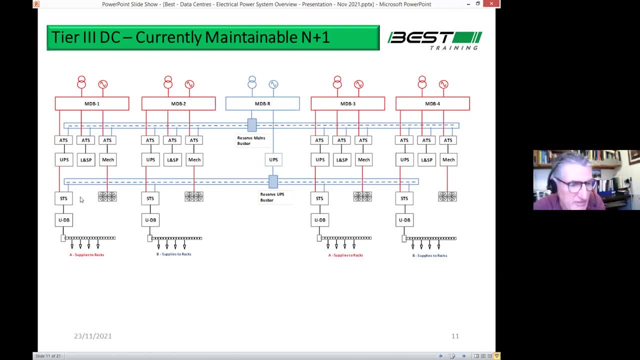 Whereas with an ATS it could be, you know, 20 or 30 milliseconds. You couldn't have that with critical load. It would see it as an outage and your servers would crash. So that's why, if you're doing this arrangement, 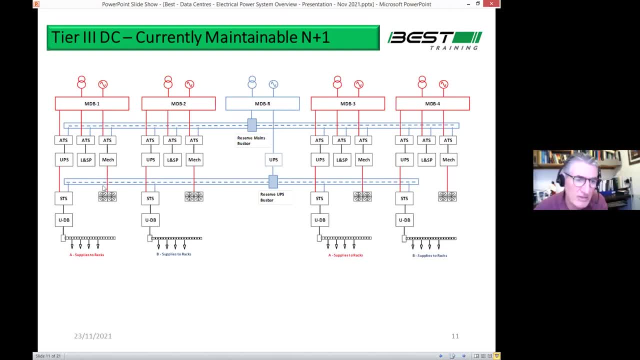 and this is not the only way. there's hundreds of different ways. This is just one example I'm giving. The critical load is able to draw its supply off this UPS or this one, So that's a typical range. We call that like a tier three data center. 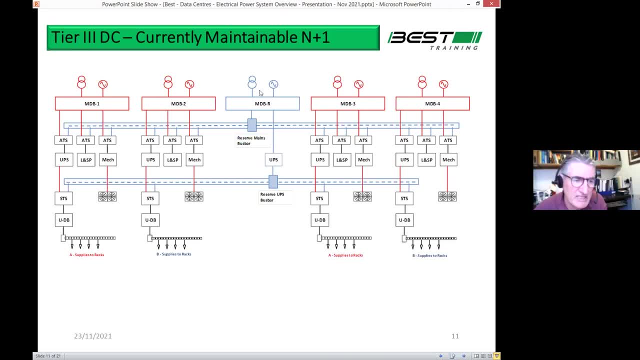 So tier three is usually what they call an N plus one arrangement. So this N plus one, which we again will cover in a few slides, means your need plus one. So this data hall here is supplied by two, three, four, five. 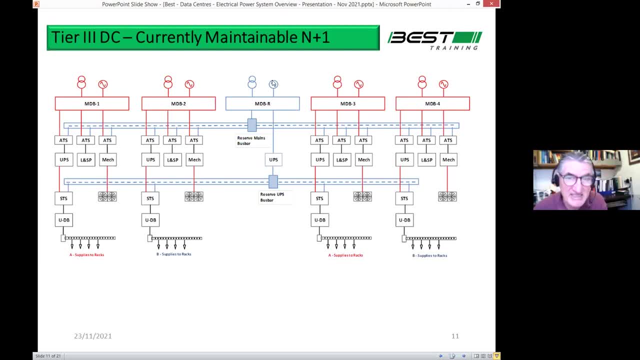 two boards- it's a need- and you have one spare system, And in this case the spare system is shared by another adjacent data hall with MDB three and four on it. So that's quite a common solution, quite a common architecture. 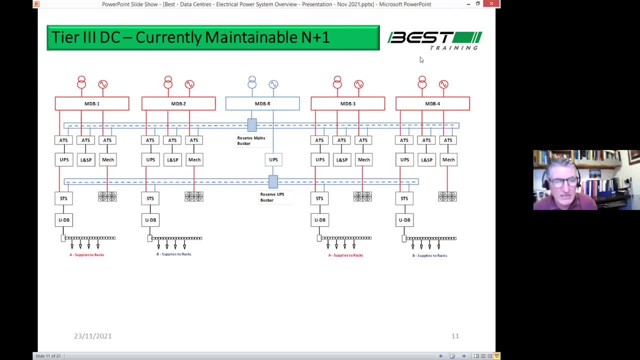 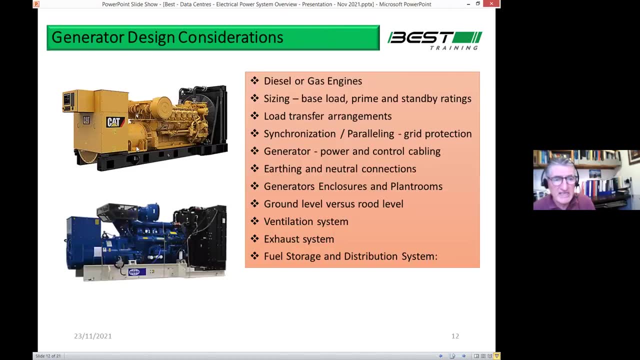 and it's probably the most cost-effective solution, And a lot of the data centers use that or variations of it, Right? so we're going to start looking at a few of the other components in the system now. So generators obviously play a huge part in data centers. 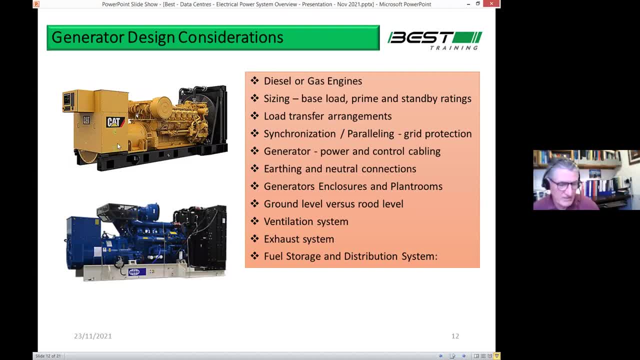 So generators obviously play a huge part in data centers And, as I said, we were informed in the Irish Times this morning that it's now going to be mandatory, but of course you take it as read. every data center has backup generators anyway. 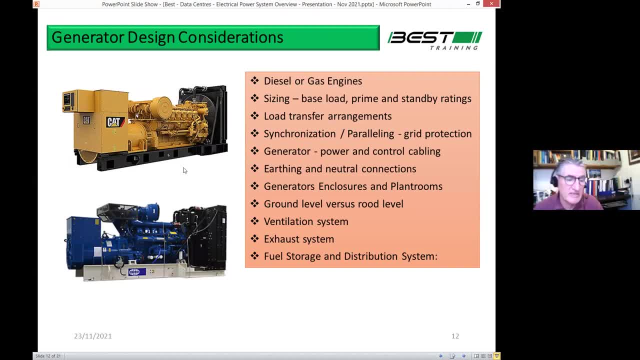 And they weren't waiting on air grid to advise them, to put them in. The big difference is they can. now air grid will be able to, by law, be able to force them to come off the grid and go onto their standby power. 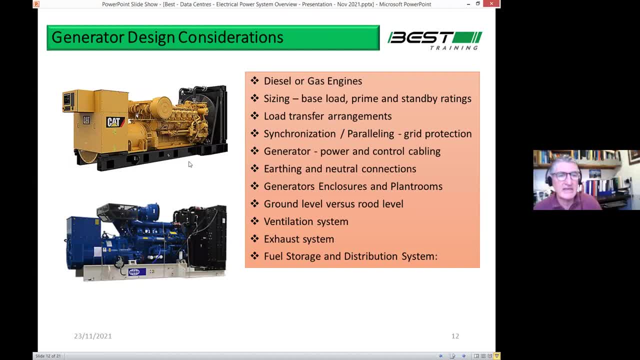 Whereas at the moment they have no obligation to do that. But I think personally. I think they will start engaging with air grid and evading of what they call the demand side management, where heavy energy users can come off the grid and assist in mitigating against risks of power failure. 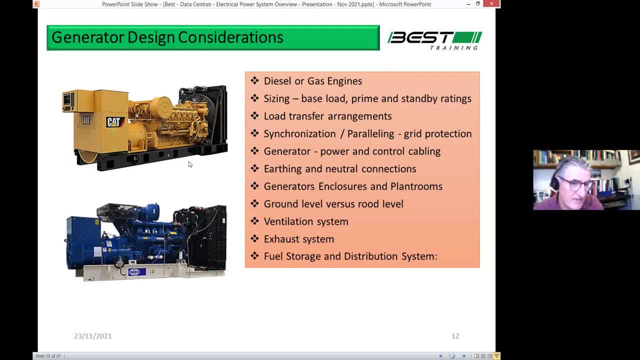 due to overloading on the grid And data centers. you know there'll have to be incentives in place, As we've had for years. we've had a thing called the Winter Demand Reduction Incentive. It's been around for decades. 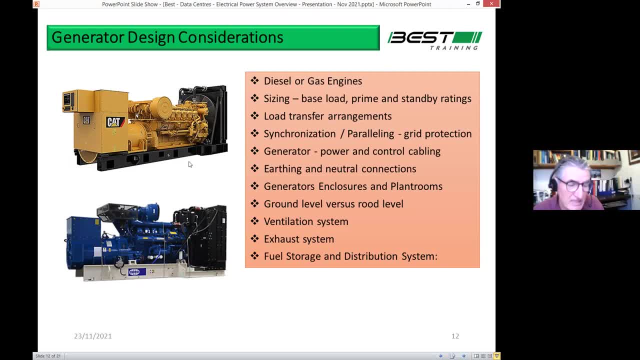 where they encouraged big consumers to come off the grid between, or to reduce their demand or transfer their demand over onto the generator between five o'clock and seven o'clock in the winter months- November, December, January, February- And by doing that, air grid. 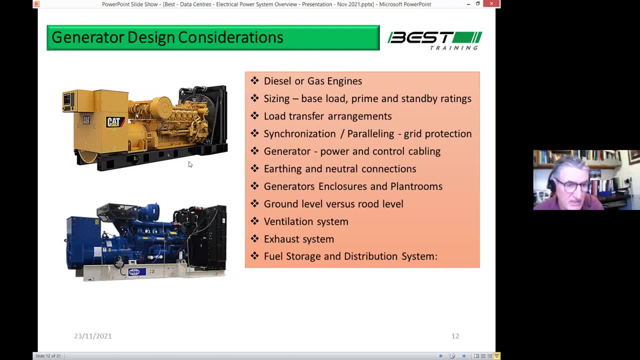 we're avoiding that big peak that occurs when we all arrive home from work. we stick on the oven and the kettle and you sit down and watch Carnation Street and you're probably kettle again or whatever you're up to, And if the demand spikes around that time, 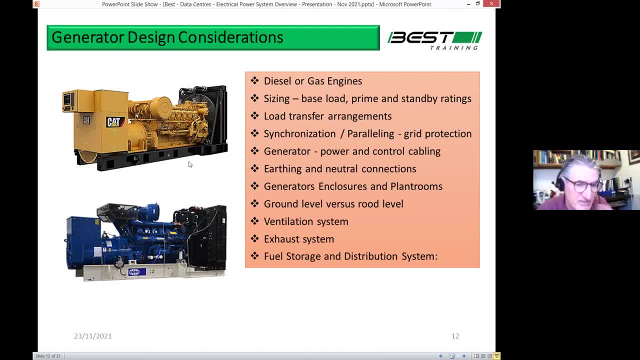 between five and seven during the winter months, and electric heaters and all that type of thing contribute to it. So they encourage people to come off the grid, get rid of that stage And that's kind of gone now and they've introduced demand side management. 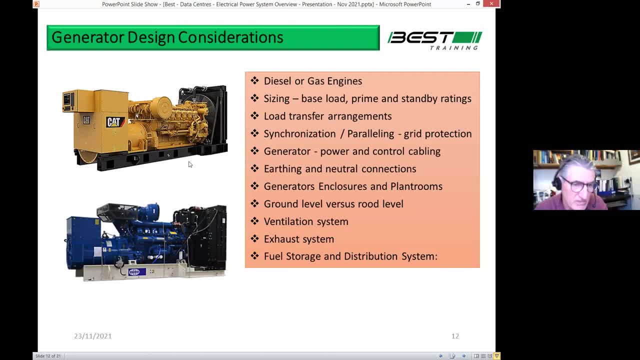 And I think they're going to have to work with the data centers and encourage them, incentivize them to start using their generators at peak periods. So there's typically what the generator looks like. It's literally just a big diesel engine. It's a V-form engine. 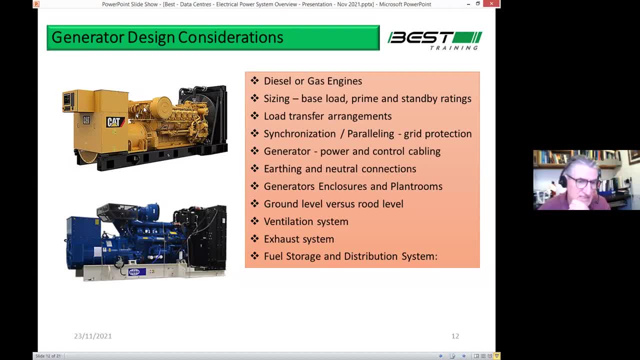 As you can see there, you can see in this one is six cylinders on one side, six on the other. So it's a 12 cylinder engine, just industrial diesel engine, And this little section in the middle is the alternator. That's where the AC current is generated. 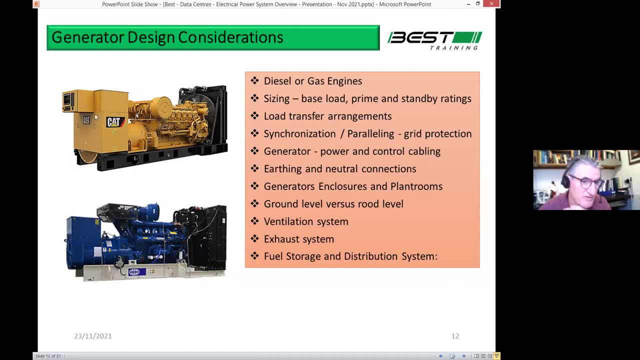 And this big box at the end is where the conductors literally come up off the alternator into the circuit breaker. And then you have the control panel here which controls same way as the dashboard on your car, you know, oil pressure, the coolant pressure. 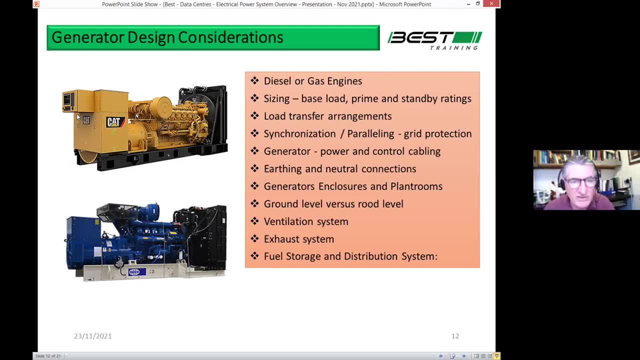 water, coolant pressure, the revs and everything of the engine. So that's all done there. And the other big thing at the end is the radiator, which keeps the engine cools and also cools the turbo air for combustion, cools down the air for combustion as well. 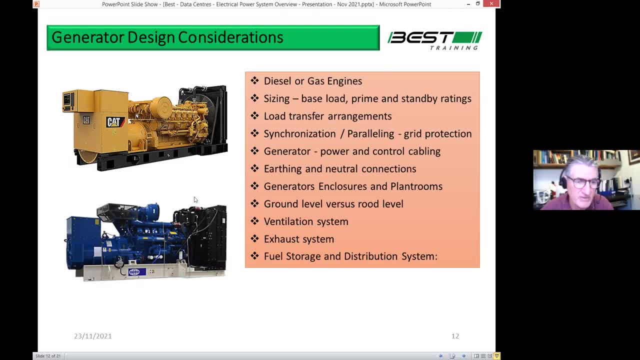 And that's a very popular made Caterpillar. We all know the Caterpillar engine's been around for a long, long time And here's one that'd been made in Ireland for decades. FG Wilson are made up in Larne in outside Belfast. 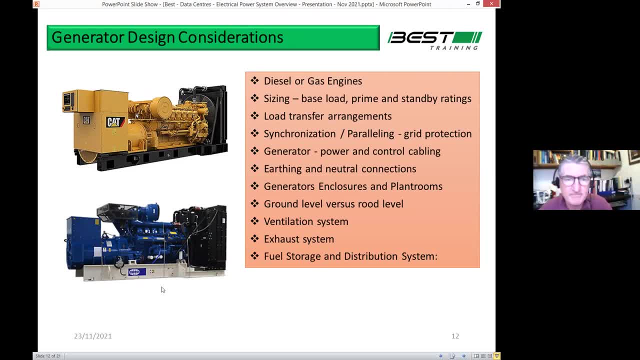 But they're now owned by Caterpillar, So they're effectively the same company. So some of the considerations: if you're a designer of a data center and you're designing the power system, some of the things you need to consider are: 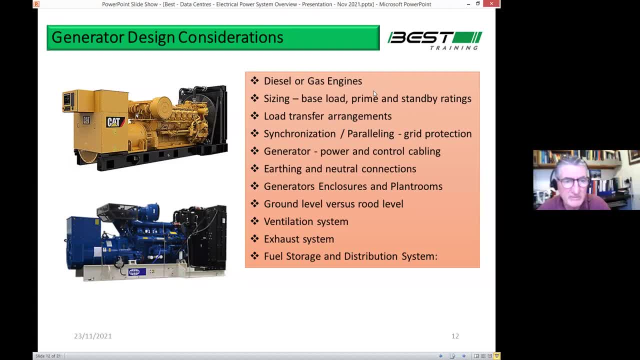 do I go for diesel or a gas engine? That's becoming more and more common If, particularly with the new data centers now, they're going to have to run for hours off the grid with their own engine- Diesels from an environmental point of view. 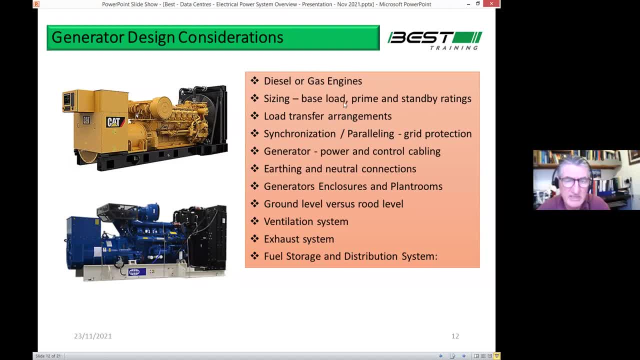 gas engine is better than a diesel engine, but there's a lot of disadvantages with the gas engine And size is going to generate where you go. base load prime or standby rate is very important. The load transfer arrangement: are you doing a load transfer? 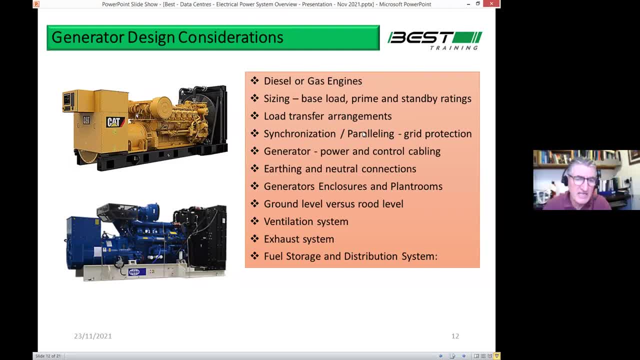 Are you synchronizing with the grid All the generator power and control cabling, how that's done, everything arrangements, The generator enclosure. do you build dedicated plant rooms? Do you put it on the roof, Do you put it down at a ground level, et cetera? 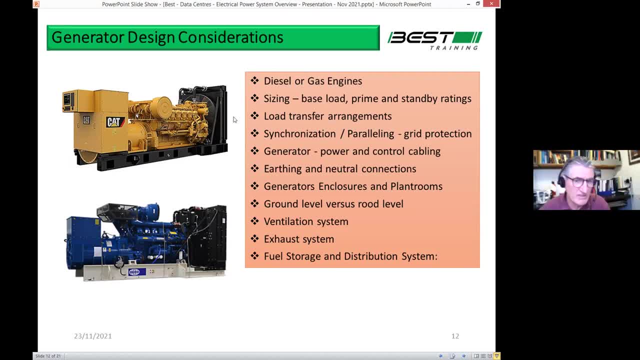 Ventilation system. they take an enormous amount of air, which isn't shown here in the diagram, So to cool that radiator down. when you're driving your car, you're driving against the wind, So the wind is blowing through your radiator and cooling it down for you. 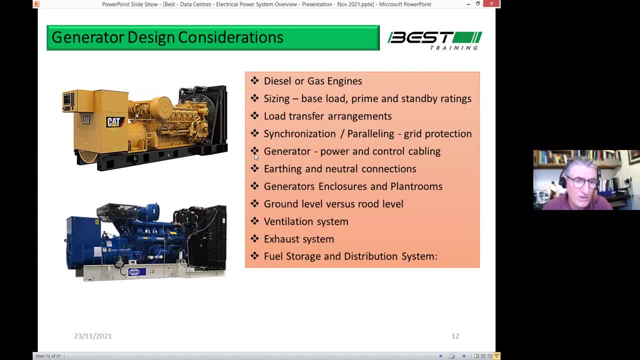 The generator is sitting in a container or in a room, So the fan has to be driven by the engine and it pulls in fast volumes of air which creates lots of noise. So you have to put it through an attenuator to reduce the sound pressure, et cetera. 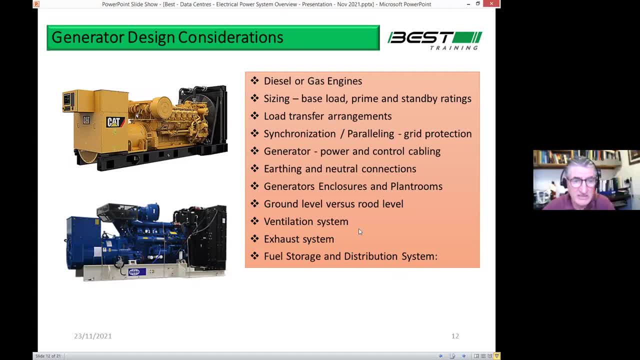 So there's lots of considerations to take into account. The exhaust system. you can see these data centers now. they're building them all over the place and they're instantly recognized by the generator flues, the big polished stainless steel flues. You see them popping up over the ridge of the building. 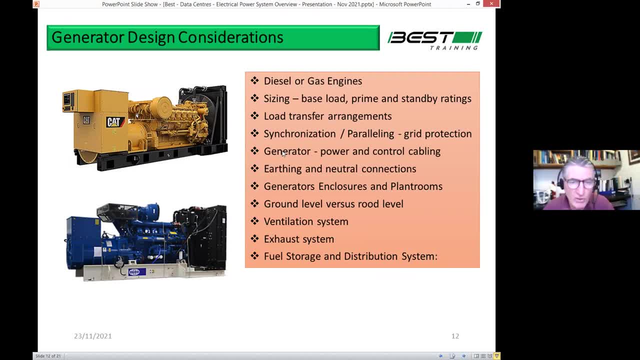 They look like warehouses. and all of a sudden you see these shiny chrome flues upside the building And it's a dead giveaway that it's a data center when you see that. So where you put the exhaust system? how you get up to the building? 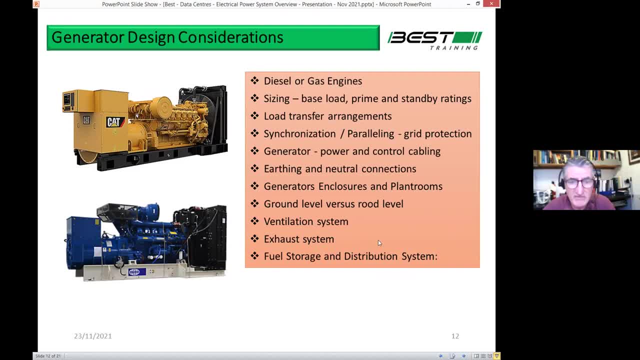 And then, most importantly, fuel storage. So your diesel generator has to have typically 36, 48 hours storage of diesel, which is a massive amount of diesel to store in the site So it can be bulk stored in a central tank and, like in a tank farmer, pumped around. 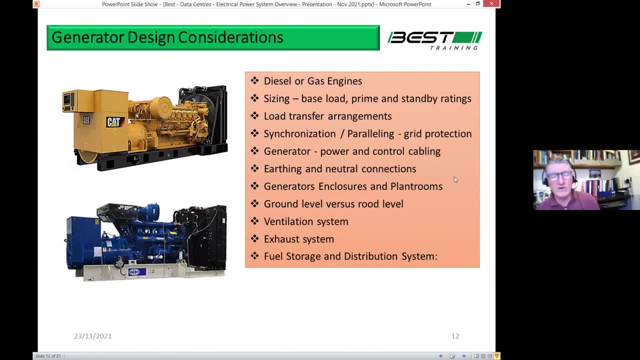 which is rarely done, not recommended, obviously, because the whole distribution system becomes a single point of failure. So the alternative is now they're building them with. each generator has a tank underneath a base tank. They're called in the industry belly tanks. 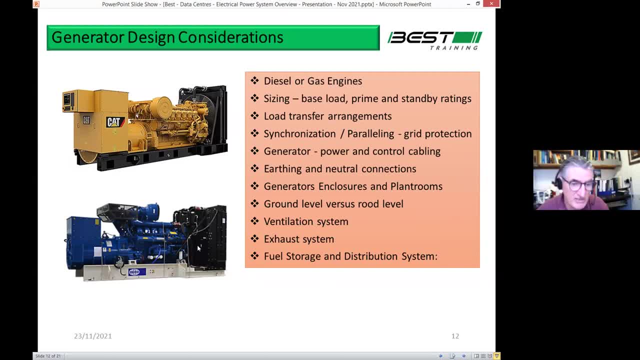 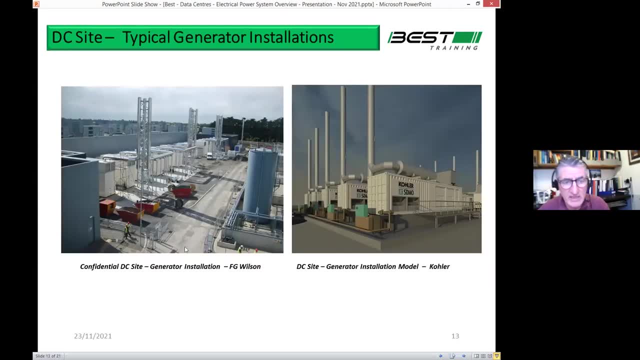 but it's just basically a big base tank sitting here and it just draws the fuel directly off the tank below it. In fact there's the image on the left is an actual confidential DC site. It's so confidential I actually don't know myself. 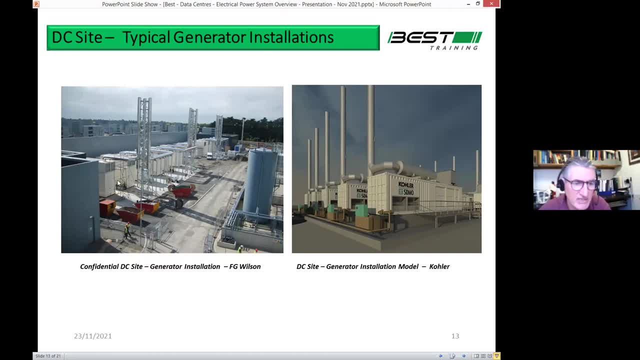 which one it was. somebody shared the picture with me, But you can see them there. They're the generators in the containers. So these are normal shipping containers and are used for roll on, roll off type containers, And you can see the flues coming up here. 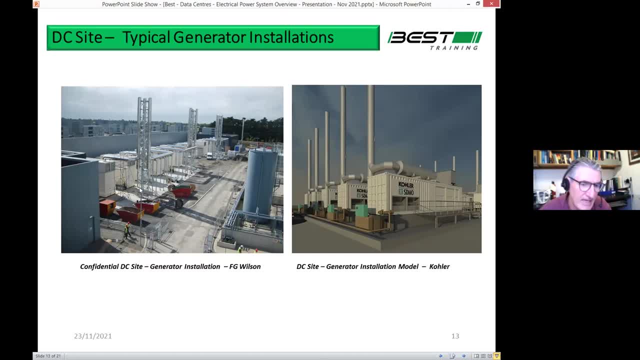 Chrome flu is going up and they're going up this stack here. that's a lattice tower like it's a triangulated lattice tower, So in this case there's one flu going up in each of the three sides of the triangle, way above the building line there. 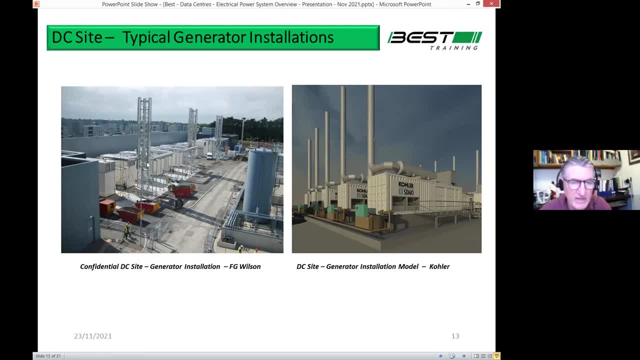 And then the next three generators goes on to the next flu stack and so on, And then you put they all go up. that's what it's going on. be fine, that's on one side, just as i showed you my diagram and then the mirror image of that over the. 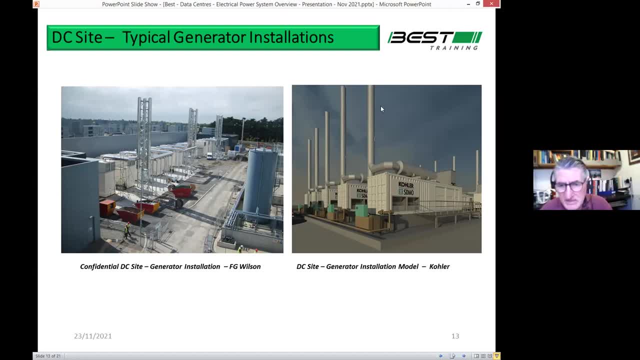 other side of the data center, and this one, i think is is a cgi, but it's. you get the drift. it's shown the generators, the flu system going up here and they see this big space down here. that's actually the belly tank on it now. so that's the container, the generator in the container and all of this. 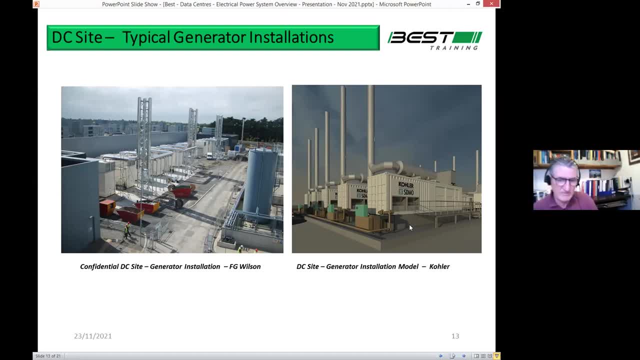 space below is fuel storage, to give you typically 48 hour storage, and the green box here is your, your field field cabinet where the fuel comes in, and that's your field cabinet. and then you have also what's called fuel polishing system there, because the fuel has to be kept healthy. and what 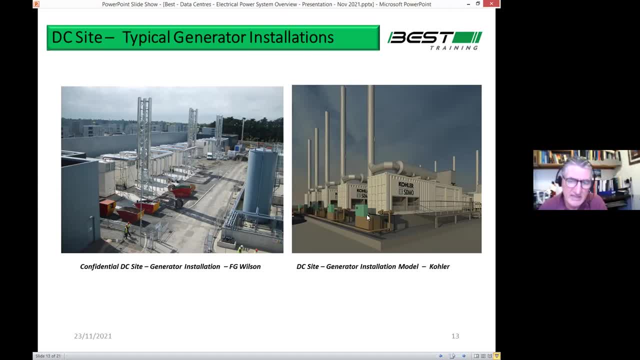 happens in in tanks is you get condensation of water and it leads to microbial growth in the fuel and it clogs up, just turns into sludge in the end of the tank and then your generator starts up, starts sucking up the sludge and blocks the filters in the generator. so to 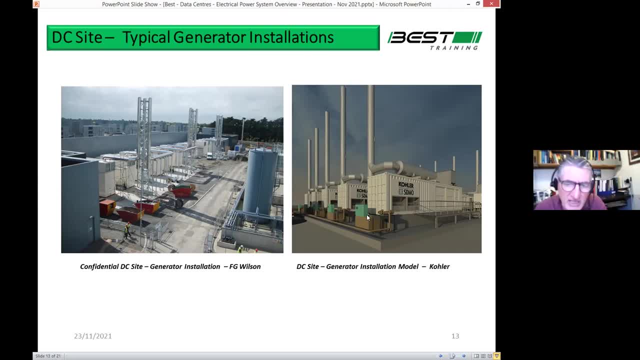 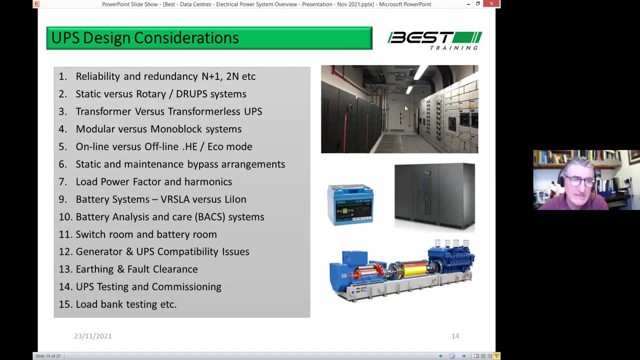 avoid that. you put in a fuel polishing system and it gets rid of the sludge in the tank and gets rid of all that sludge so it doesn't cause any engine failure later on. and next, next step down then is the ups system. so, um, so, just show you what we're looking at here. the 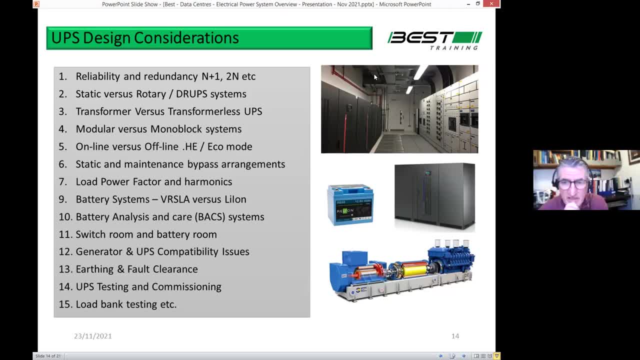 diagram. that's actually a small little data center i did about 10 years ago for aircon and that is the ups room in it. so they're the ups modules on the left hand side. so each one of those was, as far as remember was, 400 kv, 400 kva. so there's four of them there, so three plus one. one of them would have. 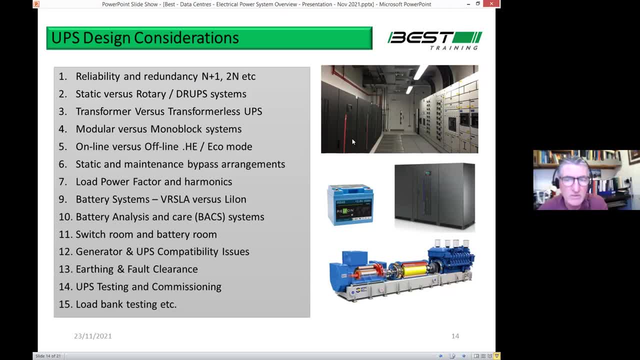 spare. so your capacity is three by 400 kva, which is 1200 kva, and then you take power, factor everything into account and it gives you about about a megawatt of power when you, when you take everything into account, and that's all the switch gear- there's quite a lot of switch gear goes into just 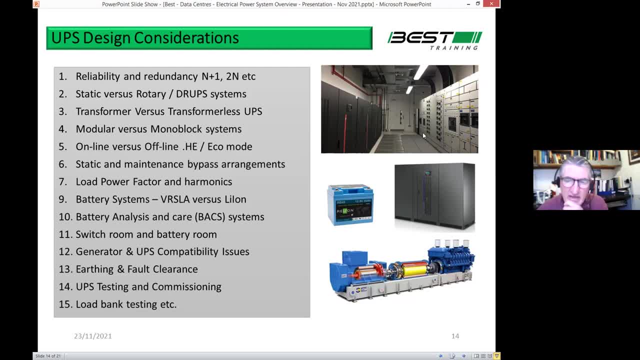 feeding those four modules: feeding the modules, taking the power back off them and then sending the power out to the servers, and that's that's the next part of our journey we're going to look at. so, in terms of ups, what do you look at? reliability and 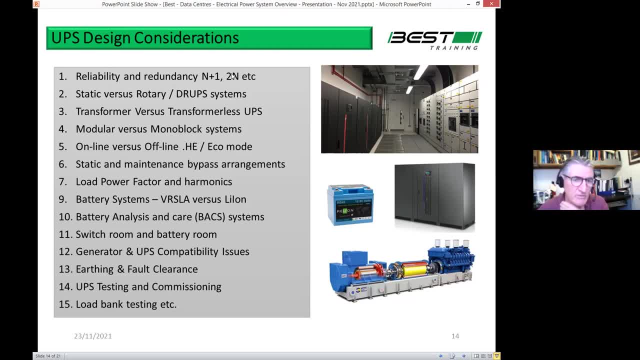 redundancy is important in all aspects of the data center, but it really comes to, comes to the fore in when you're looking at the ups system where you go for n plus one or 2n level of redundancy, static systems versus rotary. so the system in the top diagram is a static system. it's 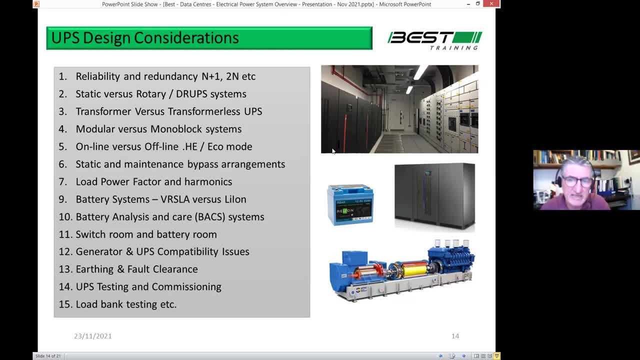 electronic components which convert the power to back to ac, and there's um the batteries, which aren't shown in the diagram because they're stored in a separate room, and the battery system is your short-term storage in a diesel rotary system, which is called a drops. is that what they're called diesel rotary ups system? 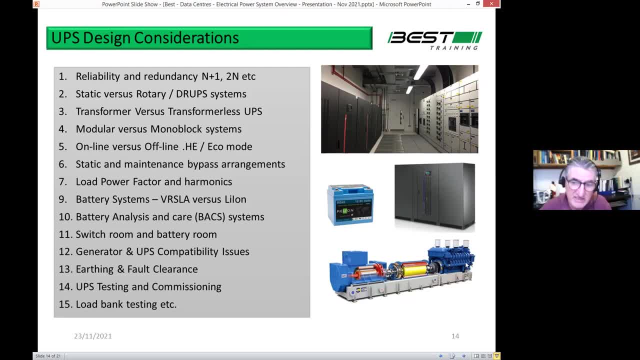 that's what you see there on the bottom diagram. so it's a generator at one end, diesel generator, as just as we saw in the last diagram, and then you have a flywheel. now i'm not going to get into explain how this works. it's very, very complex piece of uh machinery but it's basically a kinetic. 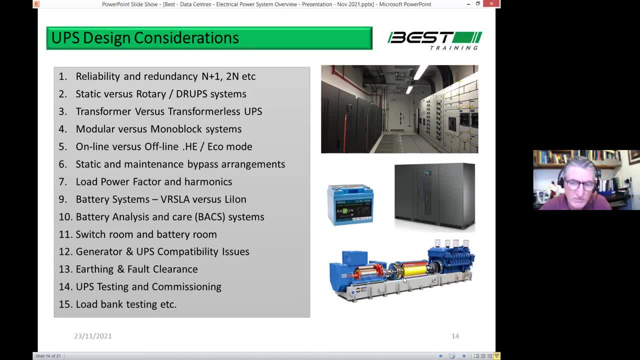 energy store. okay, so there's two rotors, one rotating at 1500 rpm and there's another one running at 3000 rpm, and that store, that's kinetic energy store. it gives you about 10 seconds- 15 seconds maybe- of energy storage to allow the diesel engine to start up so normally. 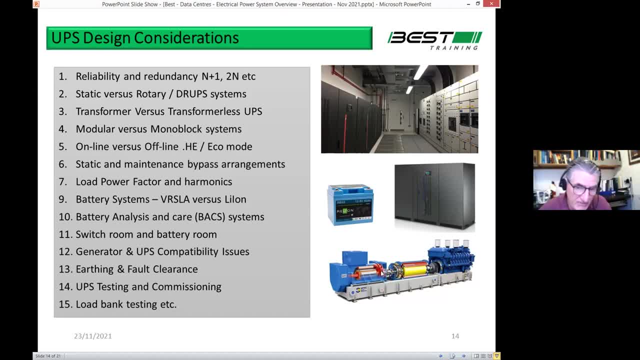 the thing is running, uh away. sorry, the motor generator part. i should have explained that at the start. the motor generator here is running away and driving this flywheel. it's spinning around and the power is going into the servers in the normal way. when the power fails, the flywheel 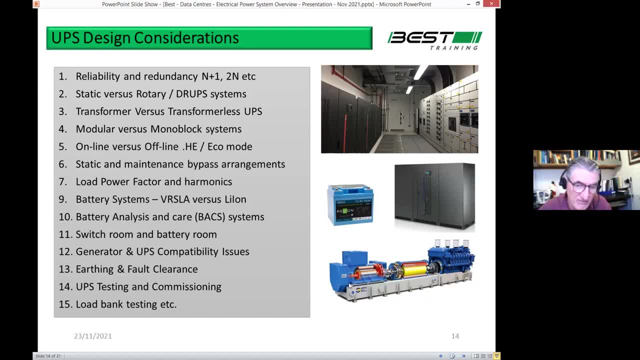 continues to run. it continues to drive the motor generator set which now turns into a generator, and the generator then delivers the power to the, to the load. so the flywheel, as i say, is about 10 seconds of 10 to 15 seconds of energy storage in it and in the meanwhile the generator. 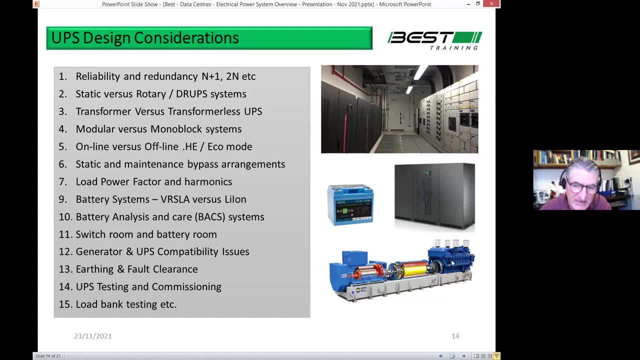 starts up a clutch mechanism, closes here and links the diesel, set back onto the flywheel, back onto the alternator and bob's your uncle. and that's how that works. so they're not very popular, so i wouldn't be worrying too much about them. 99 of the data center market, if not a hundred percent of the. 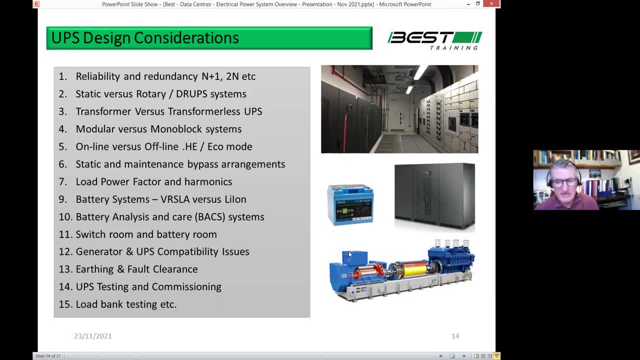 moment is served by static, and these were popular in the 90s and the early 2000s were a very popular choice, but the technology has really moved on with a static system, so they are the the main player really. so when it gets to static systems, then there's lots of other considerations. consideration: 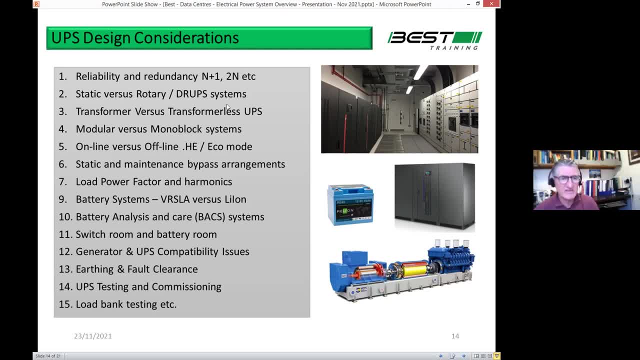 with the static system. there's transformer type systems, based transformer less systems. there's modular versus monoblock and we'll show you a slide in a minute how you operated if you operated on the line, which means you're you're sending all your power through the rectifier and inverter. 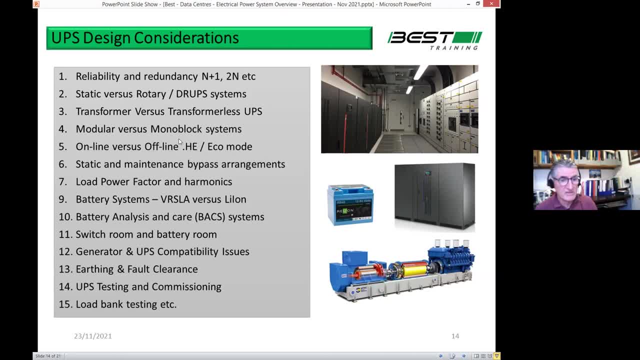 you've certain losses in the system. most uh manufacturers offer what they call a high efficiency or eco mode where you can go into, bypass and and just feed the load directly. don't go through the inverter. obviously there's a risk associated with that, but uh, the savings in. 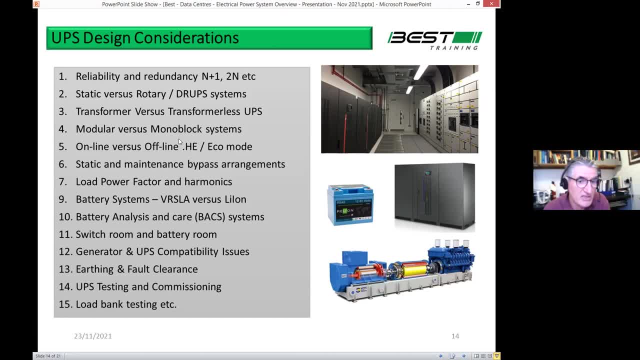 typical uh hyperscale data center like you're talking. millions and millions of euros just an energy cost per annum. millions and millions of euros just by operating in the eco mode. that's how important it is, and obviously the associated reduction in carbon emissions. there's a lot to be uh looked at there and next thing is static and maintenance. bypass how you. 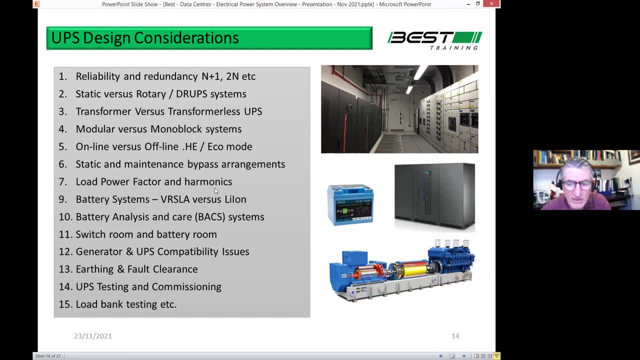 bypass the ups etc. and load power factor and harmonics etc. uh battery systems- the traditional battery is c lead acid, lithium ion is now an option and it's really taken uh gaining popularity and the battery analysis and care system, switch room, generator compatibility and so on. there's a lot to take in and there's i'm. i'm just looking at the. 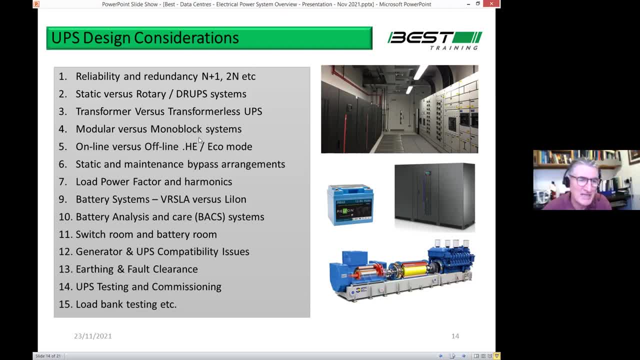 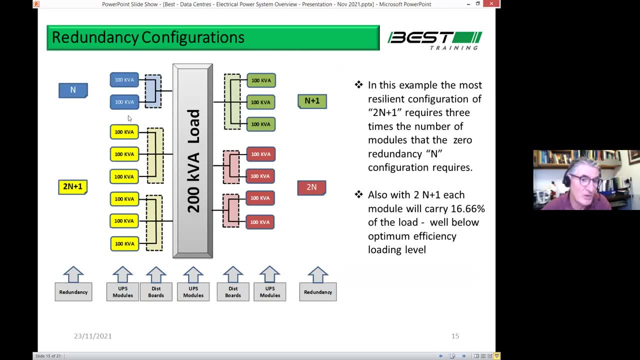 clock as well. i have a few slides to go and we're approaching a uh um question time, so i'll just move on anyway with that. this diagram i mentioned about resilience and it just shows typically here if you look top left and you have um a load of 200 kva as you see in the center. so the 200 kva represents. 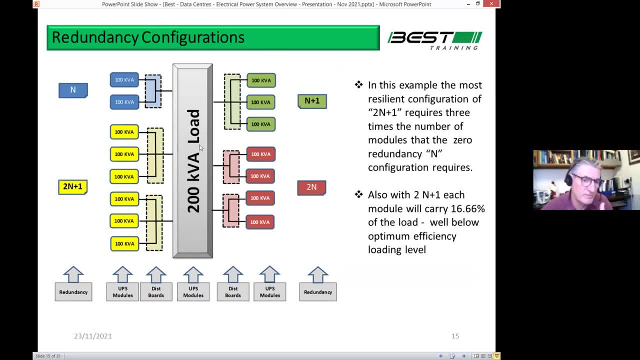 say, a data hall with a 200 kva load, which is not realistic- it would be 2000- and you decide to use a 100 kva module with a nen system, you just put in the bear two modules. okay, so you've two modules. if one of those fails, you've lost the load. so what? most data center? 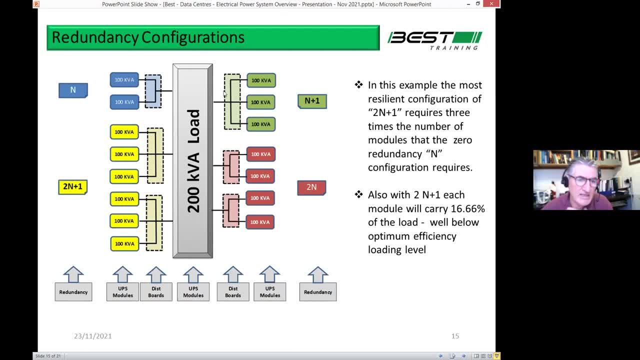 solutions. the minimum level of resilience is n plus one, so they meet the need to put in one spare module. so in this case you need three, one hundreds. two of them meet the the need and then you've won spare one. so that's where the plus, that's what the plus one means. the problem with that arrangement. 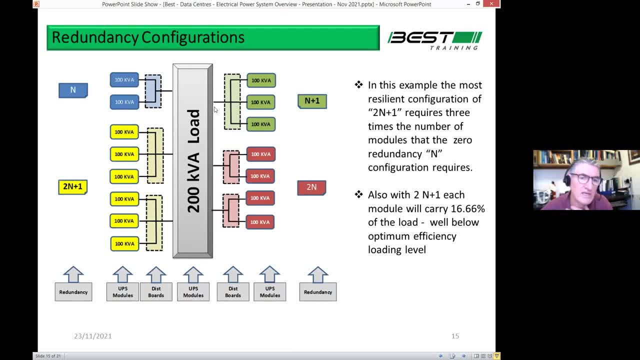 is, you still only have a single power path into the load. so if this, the switch gear associated with this ups system failed, and or the main cable- whatever on it, the bus bar system in this board failed, you would lose the entire ups system. so that's why the next one is probably the most 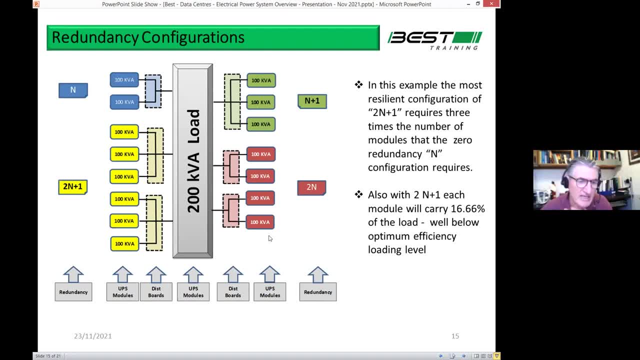 popular thing with critical loads and ups. systems are often done in a two-end configuration, which means you have an a system and a b system and both systems are capable of meeting your your needs. and a step above that that's used in some of the data centers is two n plus one, so they have an a. 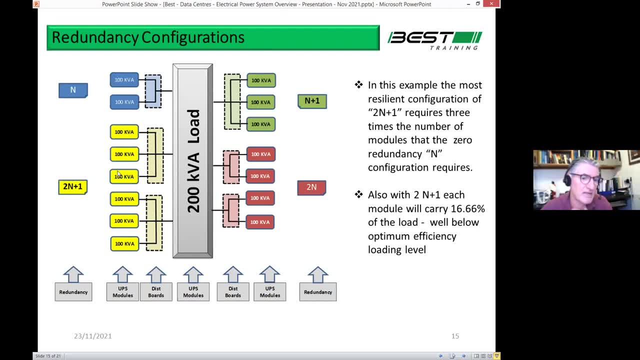 system and a b system, and in both systems they have a spare module as well. so you can see, starting off with a basic need of just 200, 100 kva modules would would meet your 200 kva demand. you end up putting six in, so there's a massive amount of additional um plan to put in data center. 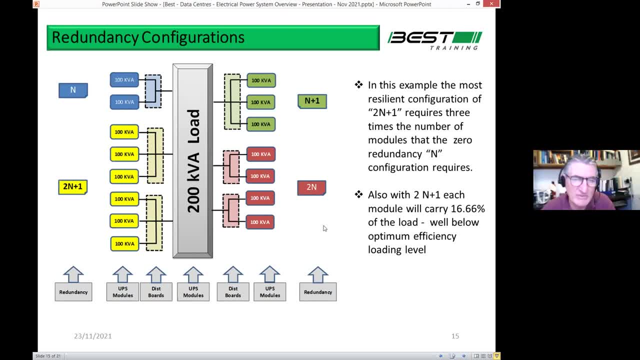 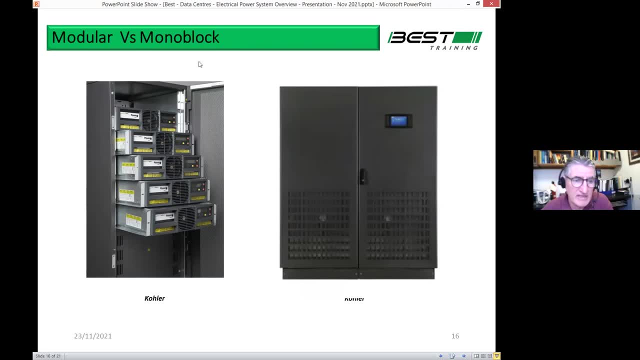 to meet this resilience element of the design. and the other thing i suggested is a monoblock versus modular. so the monoblock is what you see in the right hand side and it's sometimes called a monolith, meaning the same thing. really, it's a. 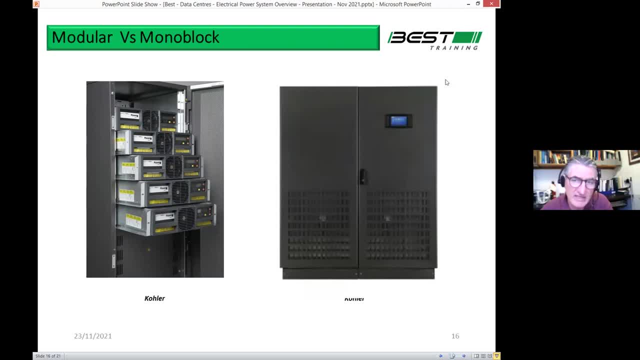 big block ups so that, for example, on the right could be a 400 kva ups system, the one on the left could also be a 400 kva ups system, but just made up of individual modules. so you can see, there there's a lot of different modules and there's a lot of different modules and there's a lot of. 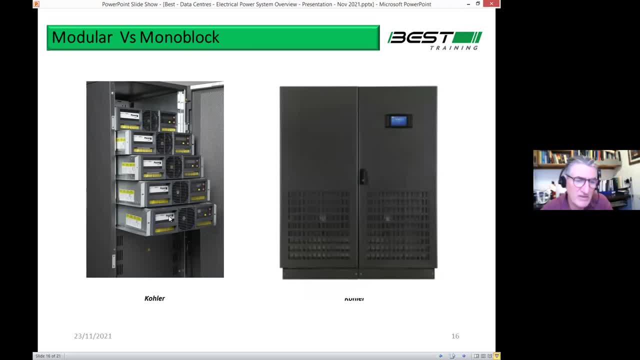 different modules: one, two, three, four, five, five modules. so each of those modules will be- let's say i'll do it the other way around, let's say it's their 50 kva, which is fairly typical. so that'd be five modules at 250k, at 50 kva, giving you a total capacity of 250 and the system on the right. 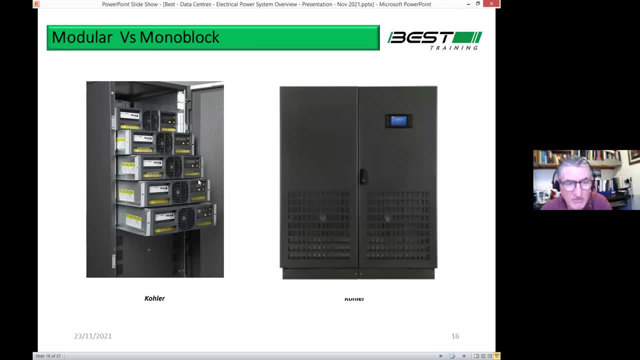 is 250 kva. so this system on the left, this modular way of doing it now, is far better. it's much more energy efficient. you can buy the modules and build it up as time goes on. uh, the availability time is much higher, which means basically, if one of these unit fails, you literally just whip it out. 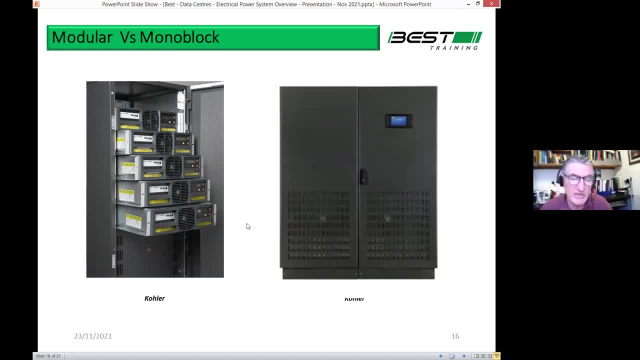 like any piece of equipment, it's plug and play. you whip it out and you replace it with another one. if if this unit fails, you have to switch the whole unit down, to start pulling parts out, like getting in it, uh, repairing your engine in the car or something. it's a fairly, fairly big job. so the 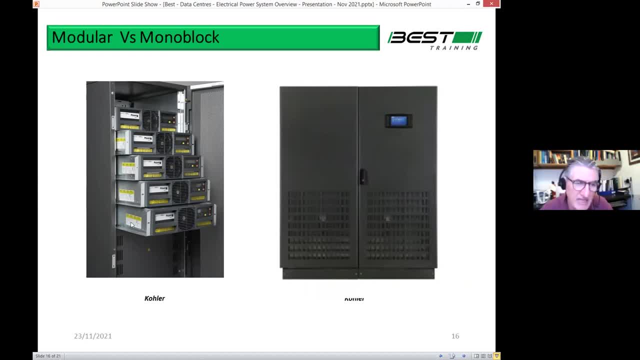 downtime it is can be much, much higher than this system and, as a result, the availability is is lower, and so, for lots of reasons, the industry is moving over to this, uh, this modular design arrangement, now and then in terms of switch gears. so the switch gear for the 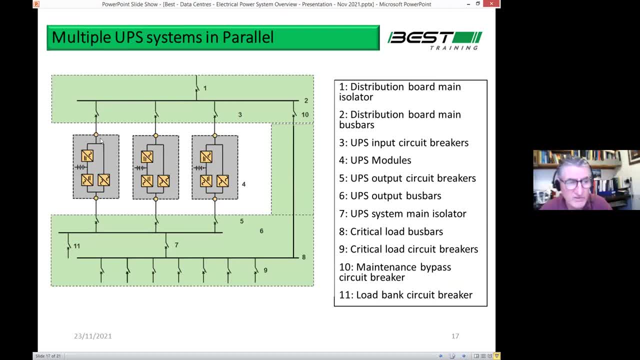 ups system is typically like this: you, this system is shown three ups systems, so it's shown in the gray boxes. so each ups system has a rectifier shown, ac coming in one side, dc out the other. then the battery connects into it there and then the inverter does the opposite of the rectifier. 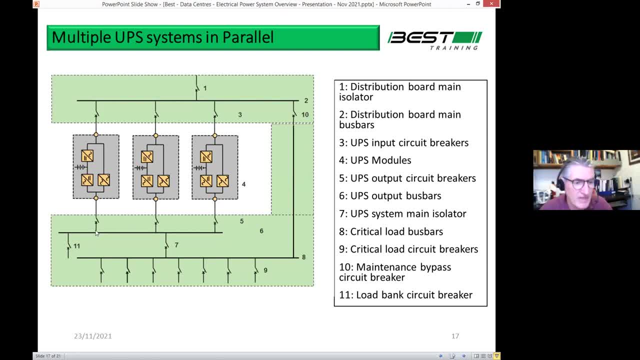 converts the dc back to ac and sends that onto the load and the other little box that you show inside the ups there with the two ac lines and if that represents what they call the static bypass switch. so if the inverter, if the system, gets into trouble or it gets overloaded, 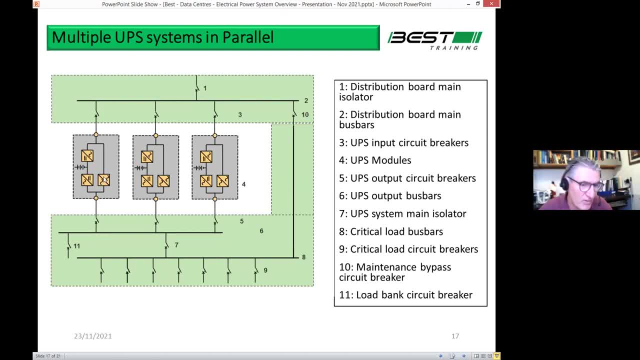 and the inverter can't handle the load, it transfers over onto this static bypass path here and allows the power to go this way. okay, so it does a lot more than apple, and that's that's basically what its function. is there that if there's a problem with this power path, it transfers? 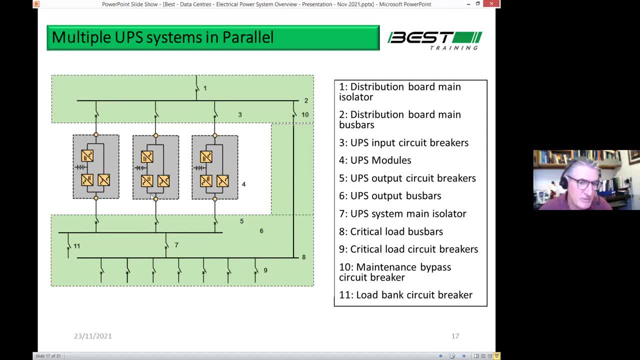 over to here. um, and this system. here the switch gear is shown three separate ups modules and you can see each one has an input breaker, on the top, an output breaker, and then item 10 has a complete bypass system on it here and then this bus bar down the end that you see all these lines here. they're going out to your 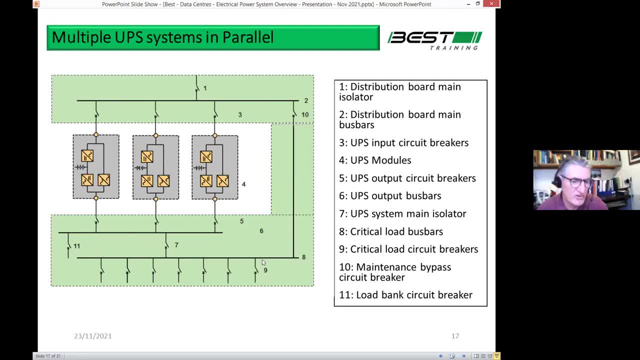 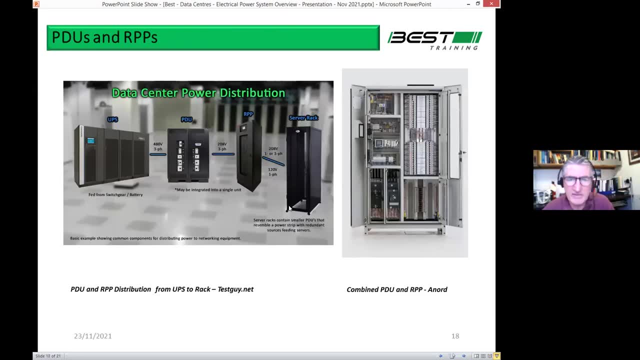 not directly to your service, that we're going out to this switch gear that in turn feature your service on our server, and that's where we're coming to in the next slide. so this is typically i found this slide and- and i was delighted to find it because it's the 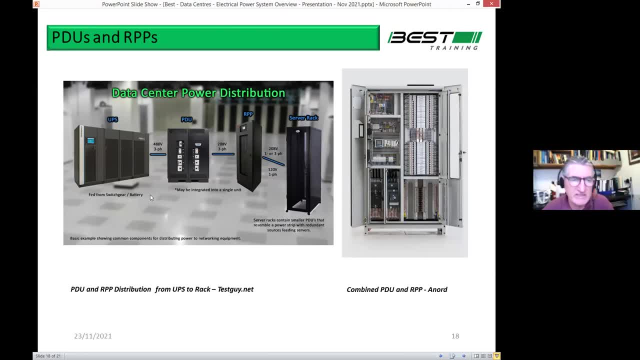 exact language i was looking for and that's the language i don't like using myself so um, but it's what's used here in the industry in ireland, because we're so uh influenced by, uh what happens in america. most of the big uh data center operators here are american. uh, as you know- microsoft, google. 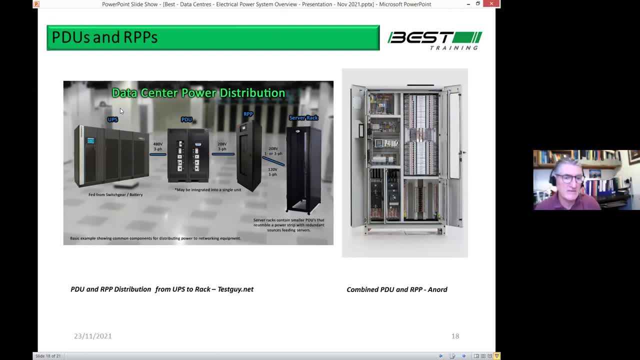 facebook, amazon are all american companies, and and many of the colo data centers are as well. they're american operators. so, um, you have the ups here, and what we're looking at is how to get power from the ups to the server. so, uh, you don't just bring big, heavy cables, you have to go through a series of switch gear. 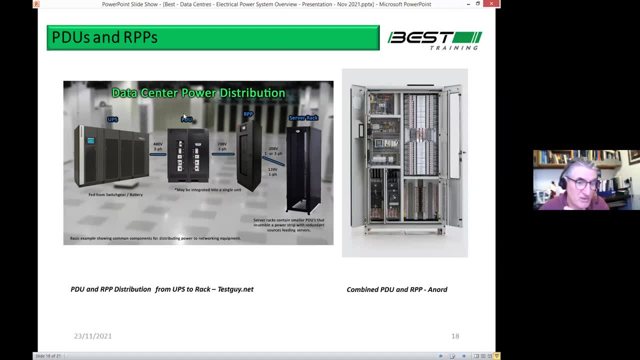 systems to get there. so in america they talk about pdus, which means power distribution units, and rpps, remote power panels, etc. the reason they do that way in america? because they have two different voltages. at low voltage they have 480, 277 is one voltage system and then they have a. 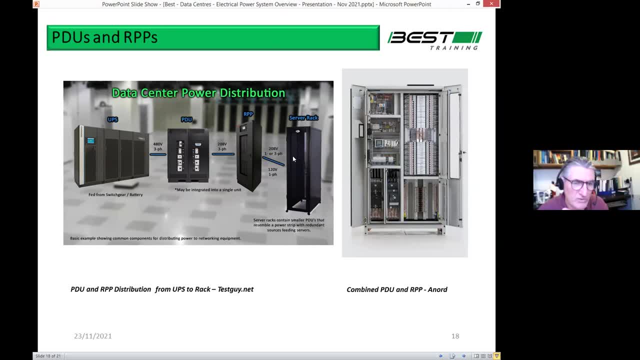 lower voltage again for smaller power, which is 208, 120.. we don't have that in ireland and and and so the pdu which has a transformer in it- we're using that term in ireland but it's not really a pdu because we don't have a transformer in it. so, um, again, i won't get bogged down to that, but that's. 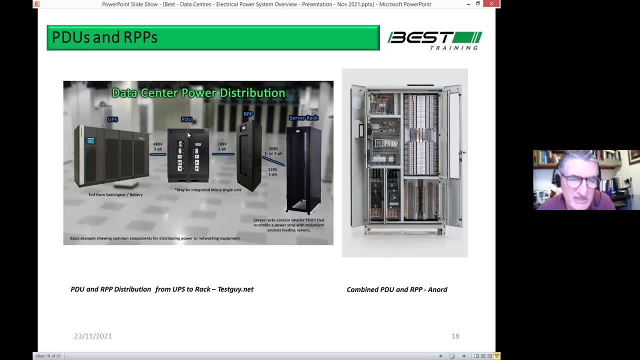 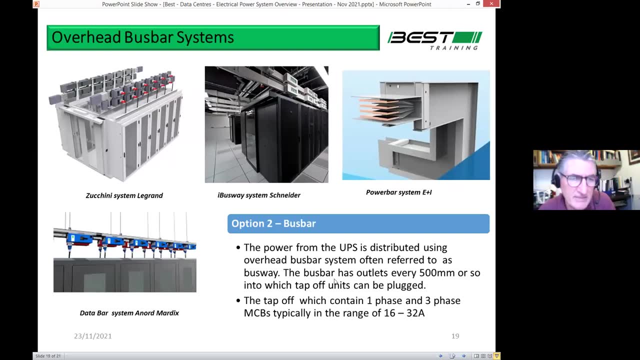 the typical arrangement. you come to the ups through some sort of a switch gear system or a bus bar system and then power is delivered to the server rack. so i'll show you in the in the next slide here typically what happens. so in ireland the most common solution is to run the power from. 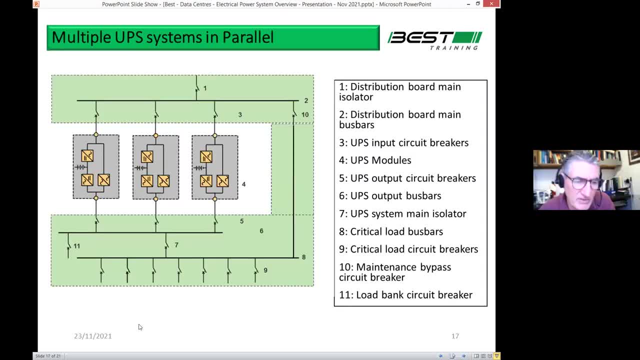 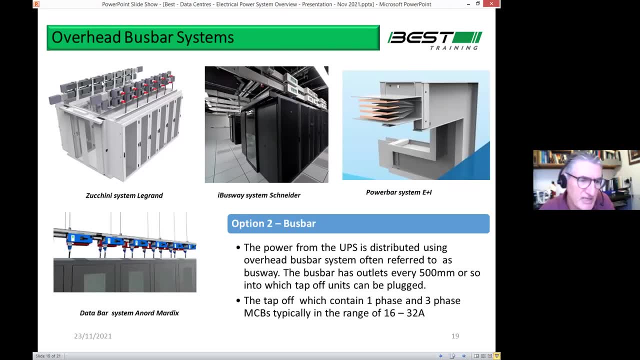 the ups system. and just to go back show you where we're talking about from these circuit cross here, item nine: each one of those would feed a bus bar system and the bus bar system looks something like this, sitting above the server racks here. so you'll see again a and the b system and you. 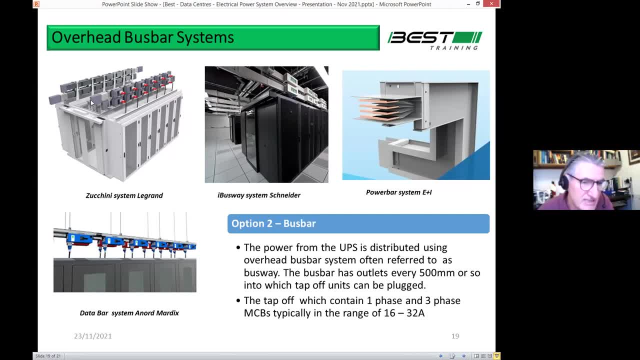 can see. the a supply comes in this end. you see the box here. the a supply comes in here, but the b supply goes in the opposite end. that's again to avoid the cables coming on the same path, to improve resilience, and then the racks on the opposite side of the pod. they have an a and a b supply as well. 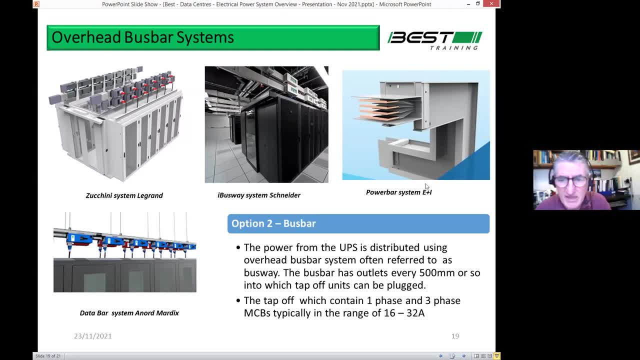 and there's some other. you can just neither have a system power bus by e and i up in donegal- really successful company just left me probably- signed the paper there a few weeks ago and a small guy, pat doherty, started a small little company 20 years ago and he sold the diverter for two billion. 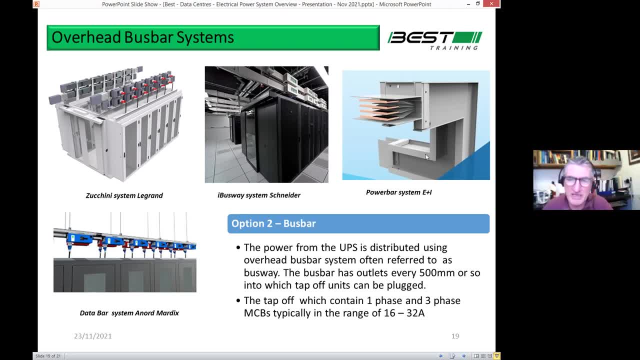 two billion euros, uh, three weeks ago, and i take my hat off to the man. fair play to him starting off from small beginnings. and that's just one of the many products that he does. and and there's another one, another similar arrangement there. you can see, this is quite. 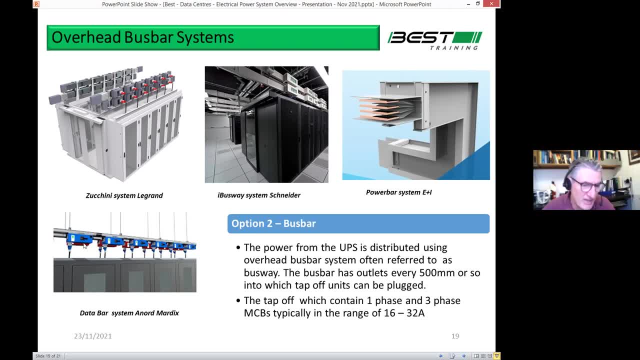 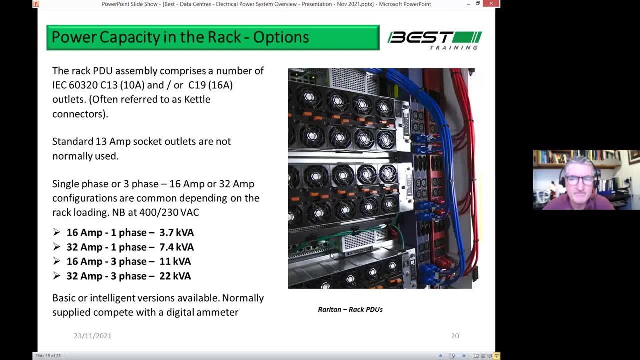 a common approach as well, the a supply being in red and the blue supply in in the b supply in blue. red and blue is often used for the a and b supplies and finally into the back of the server. we're nearly here and slightly over time, so the power comes down from the bus bar and it feeds into these power strips. 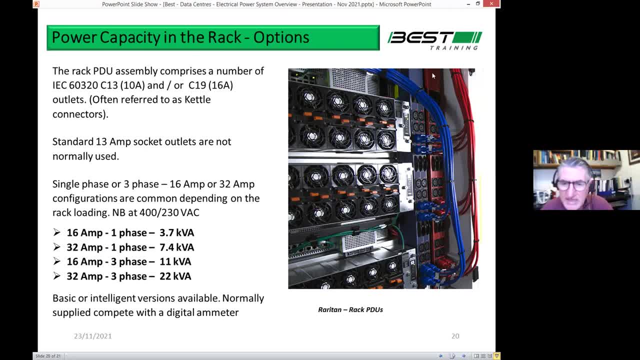 you can see them here: one is in blue again and one is in red in the back of the server rack. okay, and they are just like the multi-block you have in your desk with a strip of sockets. it's an intelligent version of that. okay, so i'm going to show you how to do that in just a moment. okay, so i'm going to. 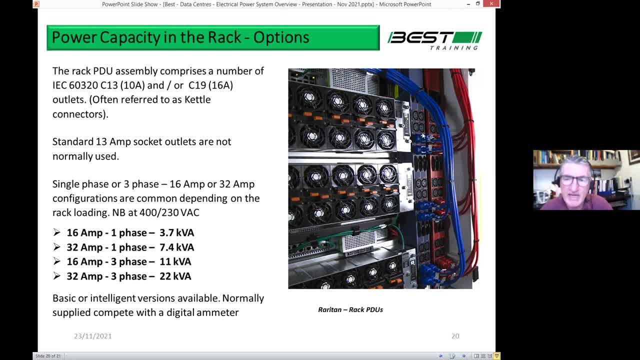 show you how to do that in just a moment. okay, so all the sockets are monitored and everything the power can be measured through them, and then you take a red lead and a blue lead up to every server. so every single server has a um an a supply and a b supply to it, and they can come in single.